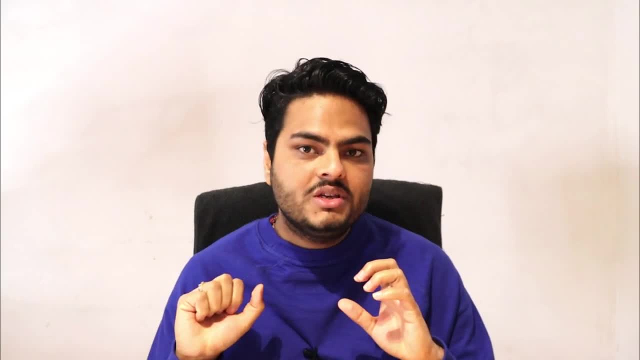 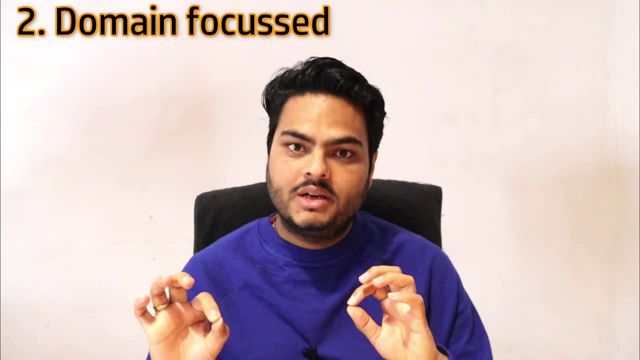 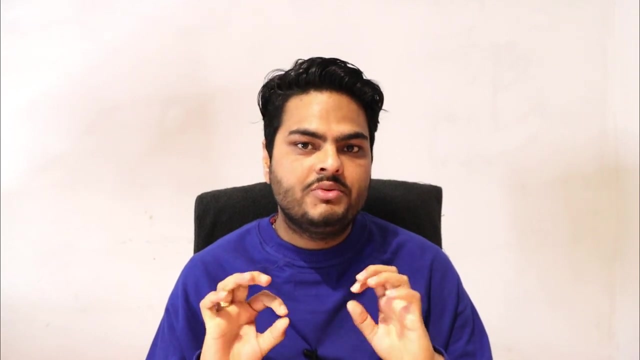 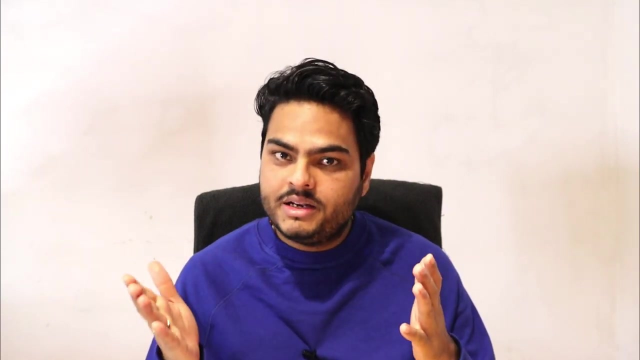 In data science. there are knowledge areas which is heavily statistics focused, There are knowledge areas which are heavily domain focused and there are knowledge areas which are heavily IT focused, and cloud technology is one such area which is very, very heavily IT focused, and that is the reason many people coming from different background than IT do not feel quite comfortable with cloud. 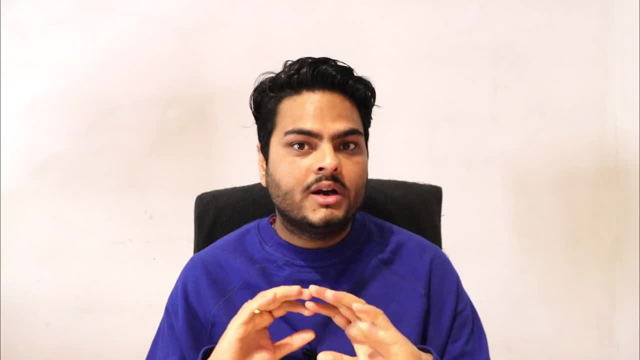 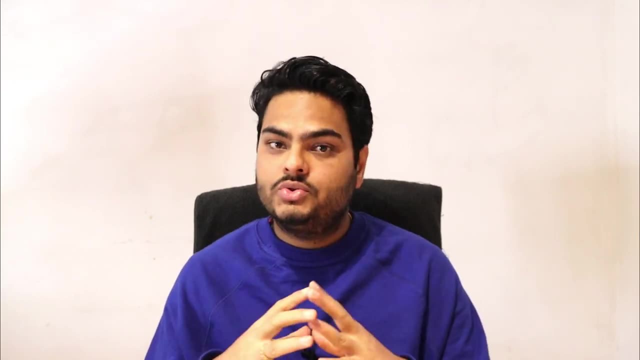 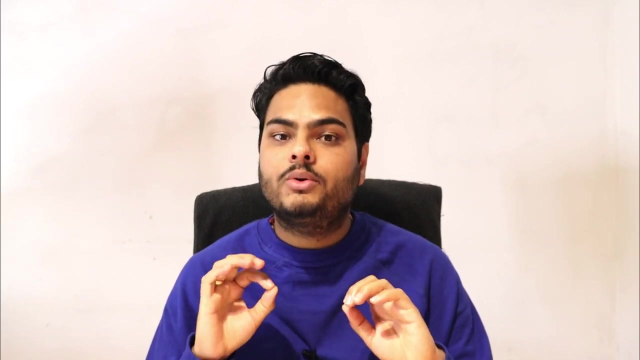 technologies. Okay, and let me tell you guys, gone are the days when you say in an interview that, well, I don't have any exposure to cloud technology and still you used to get a job. Nowadays, in good organizations, your resume may not get shortlisted if you don't put cloud. 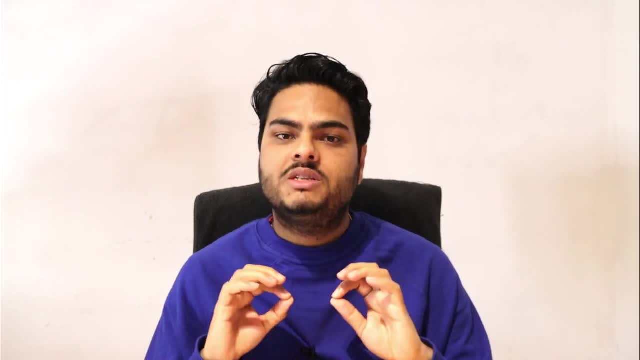 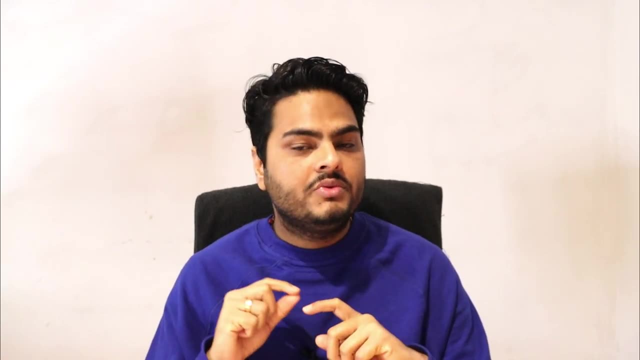 technologies at all. I am here to solve the same problem for the people who find it very, very difficult to learn cloud technologies. I am going to create a series of videos which will help you too. I am here to solve the same problem for the people who find it very, very difficult to learn. 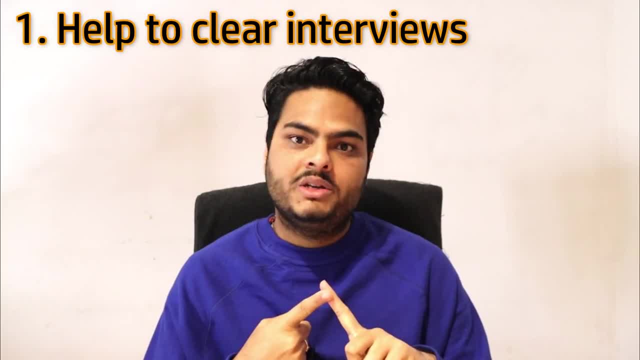 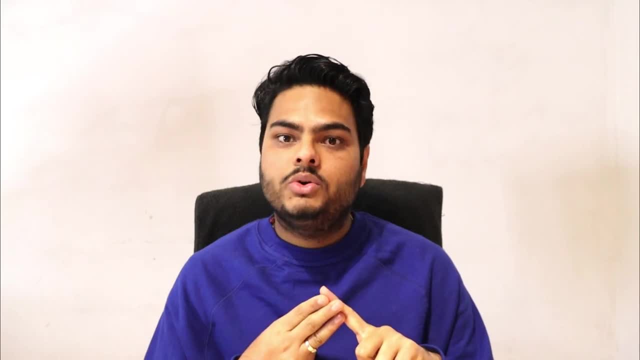 cloud technologies. I am going to create a series of videos which will help you too. Number one: clear interviews and answer cloud based questions. Number two: getting your hands dirty with AWS. and number three: building, deploying your models and how to use various components of. 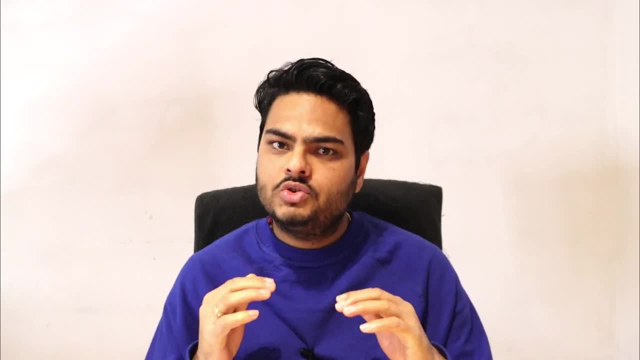 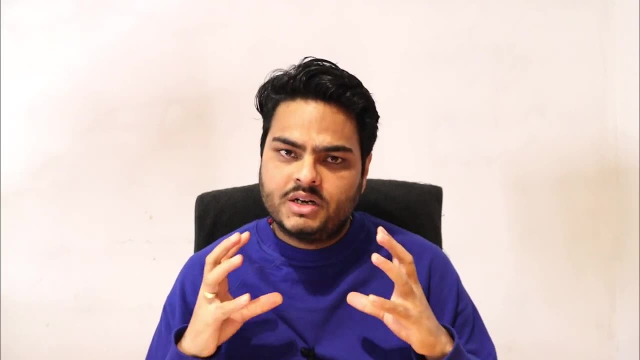 cloud technologies: How to be quite comfortable so that tomorrow, in a project you are given a cloud project, you are quite comfortable to work on. that. Let's see one by one, guys, and let's start with the basics video first. In this video we are going to learn about basics of 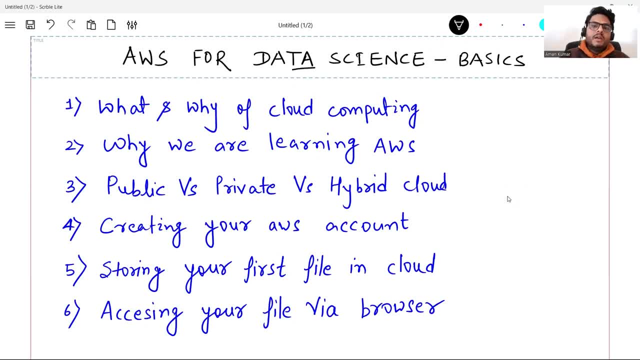 AWS for data science. okay, and what are the topics we are going to cover? we are going to see what and why of cloud computing. non-bookish definition, not the bookish definition. okay, then, why we are learning AWS, why not GCP or Microsoft Azure? I am going to tell you that public versus private. 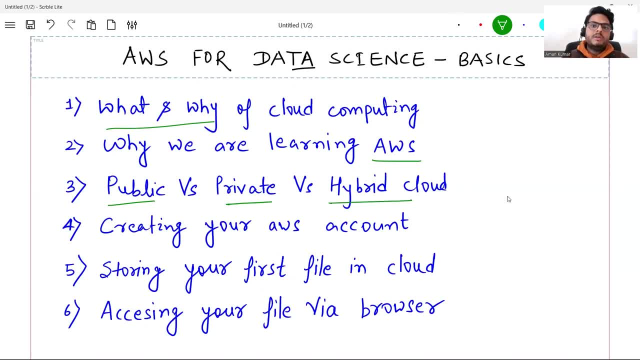 versus hybrid cloud. what is the difference? very, very important- and interview question: how to create your own AWS account. many people have confusion around this and I will show you how to create it, storing your first file in cloud. how to do that very, very easily- I will show you- you can do it parallelly with me- and how to access your file via browser. 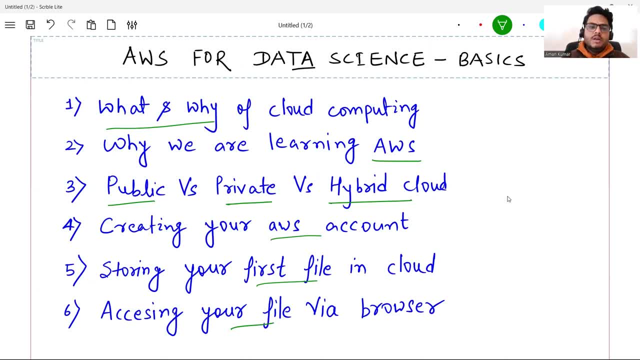 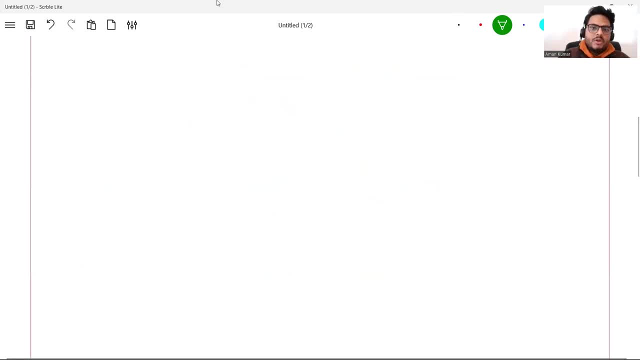 that you have stored in the cloud. okay, AWS cloud. let's see all these one by one, guys. first of all, what and why of cloud computing? pay attention here, guys, this is a non-bookish definition, very, very important to understand. okay, so I will not take any other example. I will take my example. 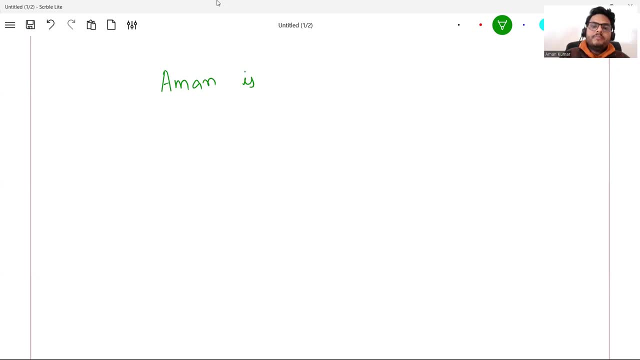 so Aman is a data scientist- okay, Aman is a data scientist. Aman wants to create one or two data science courses- okay, and he wants to host it somewhere. so currently there is a website called wwwunfolddatasciencecom. okay, so you can open it in browser. I am going to show you also. 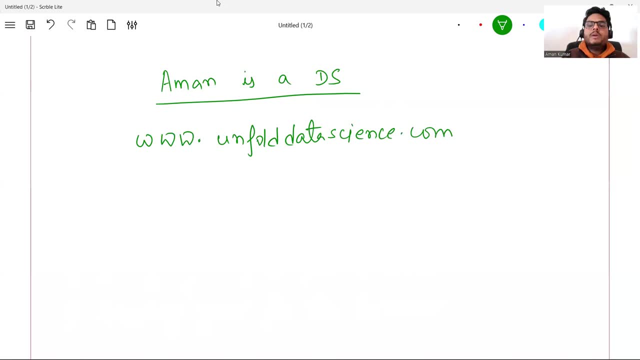 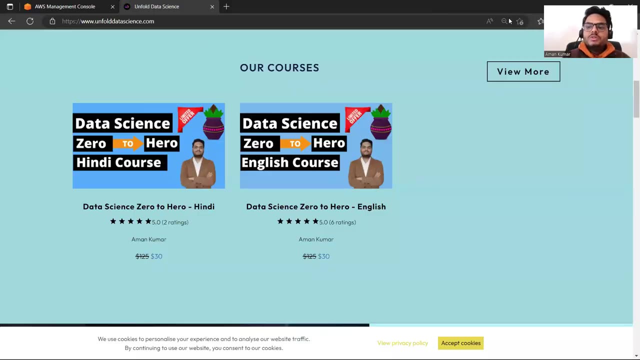 this is to relate: why do we need cloud computing? okay, so this is the website: unfolddatasciencecom. let me go to that website and show you how it looks like. so this is how the website looks like now: unfolddatasciencecom. 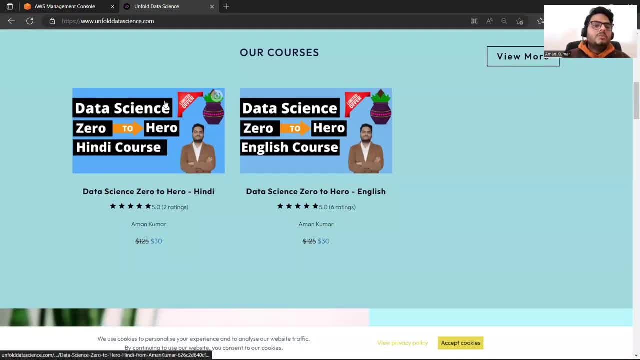 and I have couple of courses here. so what is happening right now is, for a moment. just think that there are 10 students who have purchased this course. okay, but tomorrow I don't know if 10 students or 100 students or 10 000 students will purchase my course. okay, that is my problem, number. 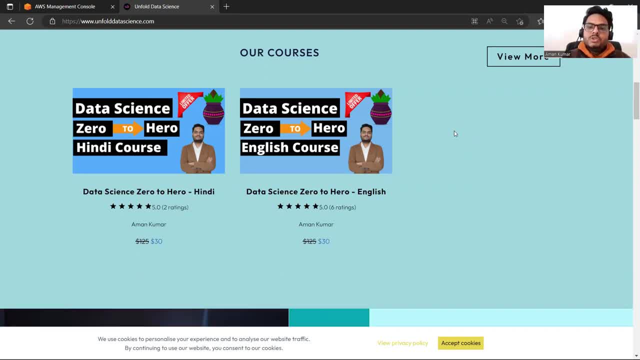 one problem. number two is: I want to ensure that nobody should be able to download this course and use it in a wrong way. I mean resell it or something like that. that is the security part. what is the third part? I want to be ensuring. I want to be ensuring this course is available in. 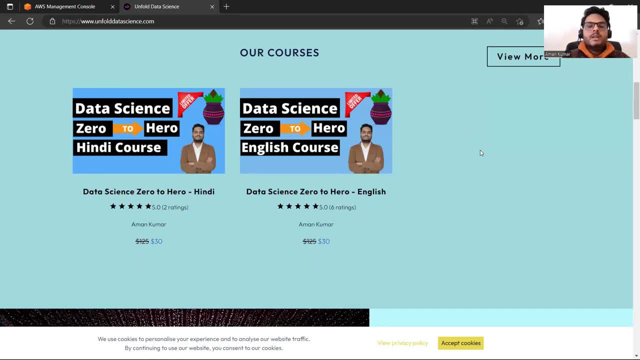 India, in USA, in Australia, in London, in, let's say, UAE, all the geographies. this course is available and same content, same latent, and the same content, and the same content and the same content and the same- I mean low latency, same kind of quality in terms of video- is available at all the locations. 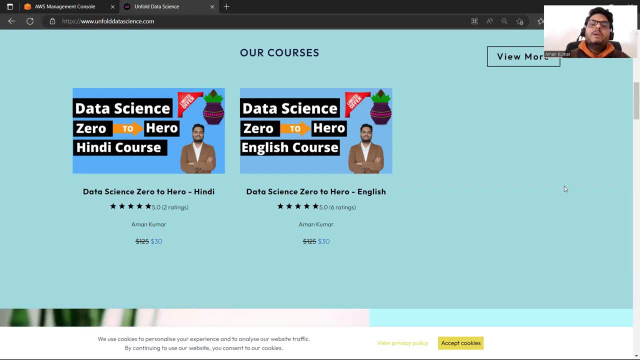 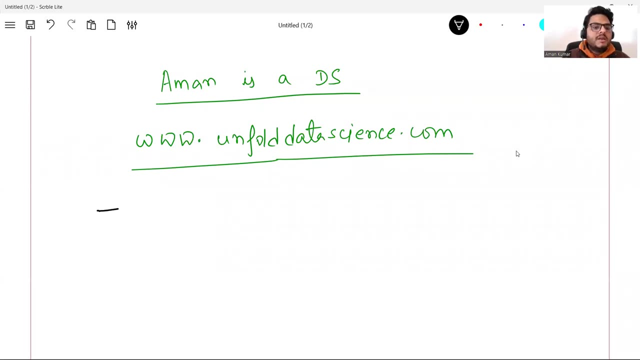 okay, and I want to ensure that if I want to migrate my entire thing to some some other platform tomorrow, or if I want to host it to somewhere else, that process should be easy. I have explained here four things, guys, what I explained you. the first thing I explained you is scalability. 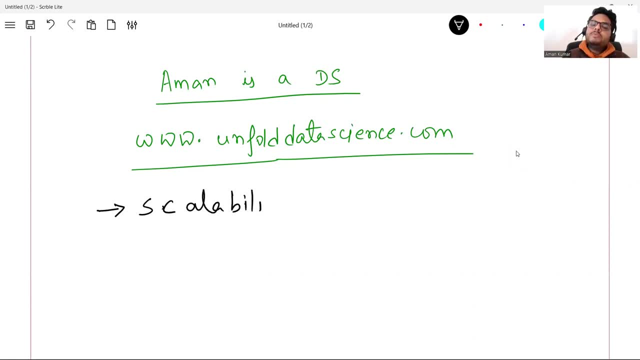 okay, so that is my first need. why that is my first need? and that is because now, let's say, 100 students are buying my course, tomorrow then 10 000 students, god knows, tomorrow one million students may buy my course. so my platform should be able to support. 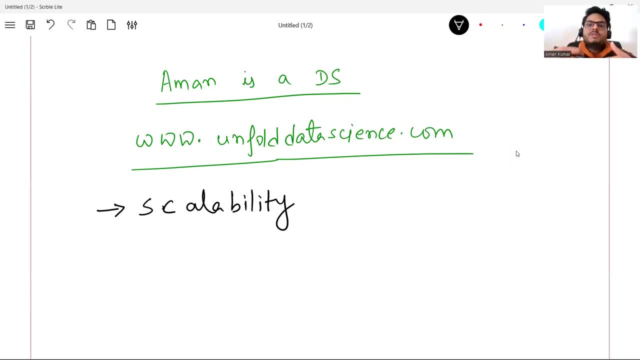 for that? I should scale up my backend, right? I should scale up my server wherever I am hosting. my course that platform has to be scalable. okay, then I told you it should be secure, okay, so that nobody is able to use it in a bad way. nobody is able to download it. 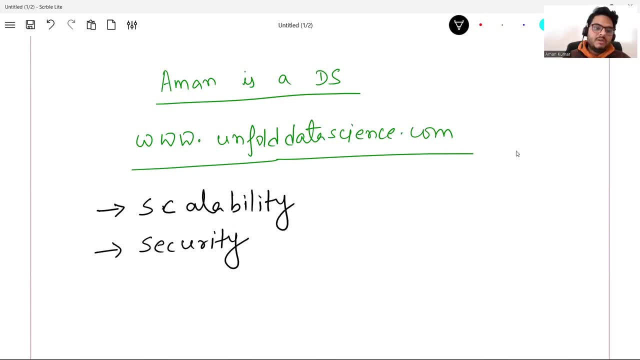 resell it, all those kind of things. security comes there. then comes flexibility. flexibility means: tomorrow I want to use it in some other platform, or I want to migrate my courses, or I want to add a new chapter, new module, more you know data examples, more python notebooks or more programming. 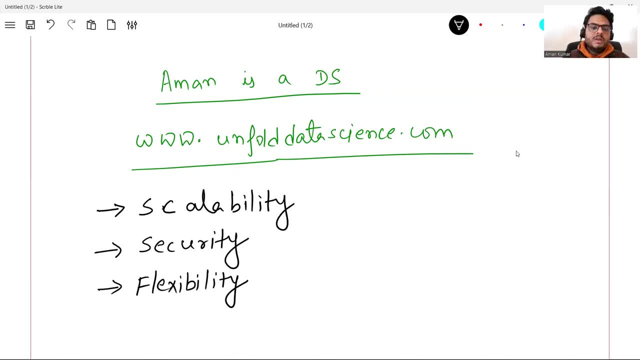 examples. whatever it is, it has to be flexible, okay. and then I told you it should be accessible in UAE, India, China, Australia, Australia, USA, UK, all over the globe. it should be accessible, so it should be reliable. okay, now understand my problem, guys. I am a one person, okay, I don't have a team, so I am the one who is. 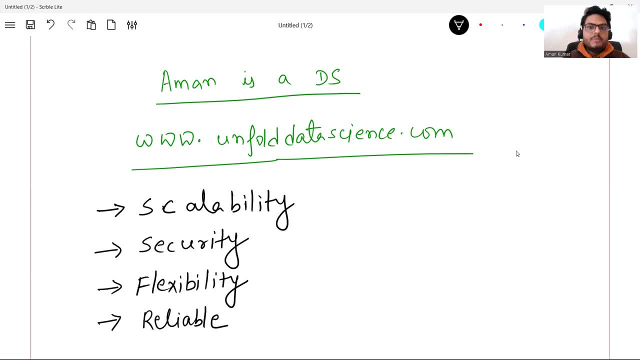 creating the courses. I am the one who is hosting that on the on that server. so you know, from your, from your normal understanding, you can think that I should focus more on creating good content code or I should focus more on these things. both are equally important, but where is my expertise line? 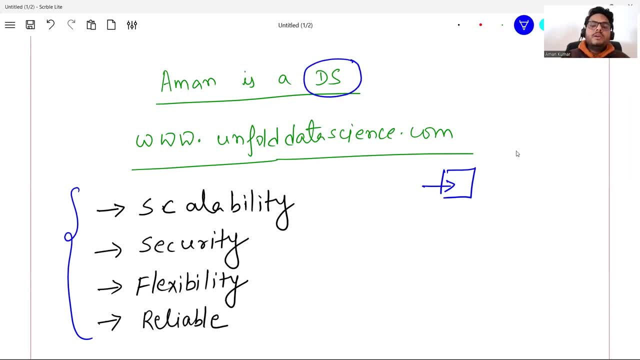 my expertise is lying in data science, right, so I can create very good quality courses in data science, but I cannot ensure all these things because you know that is not my expertise. somebody else should take care of that, okay? and all these, all these things are needed in my business, so you can think. 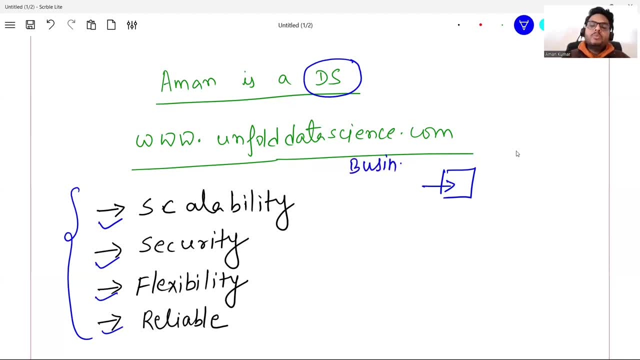 this is a business where you know one thing is product, one thing is what is my business? so my business is, you know, creating courses and hosting it somewhere, but there is it part of it as well. it part of it means it should run in a smooth way, it should be available, it should be secure, it should be reliable. 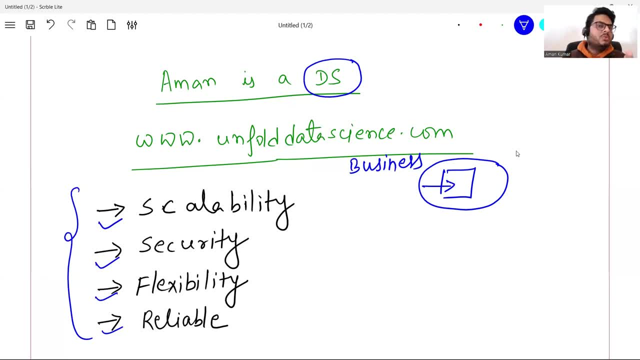 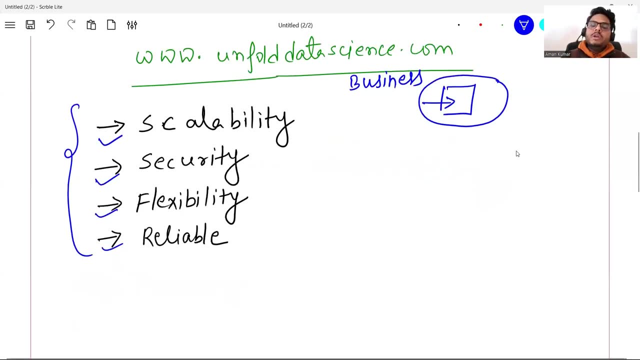 okay, and here comes the non-bookish or non-formal definition of what you hear as cloud computing. so what cloud computing tells you is: you take care of your business, all your IT to me. you give me some money, I will take care of all your IT part. so everything here. 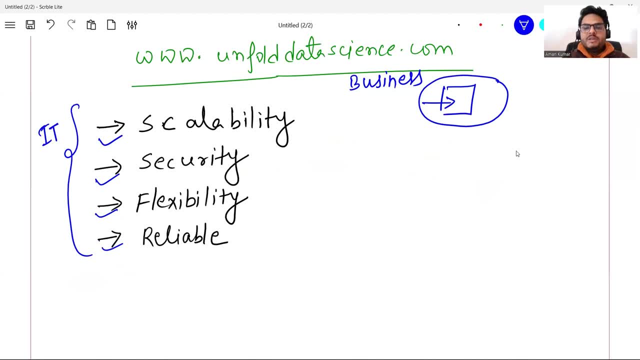 is IT. okay, everything here comes under the IT management or IT infra or IT side of the business. you can see, this is the product side of the business. okay, this is IT side of the business. now imagine here I spoke about one simple course. okay, suppose you talk of big, big organizations. 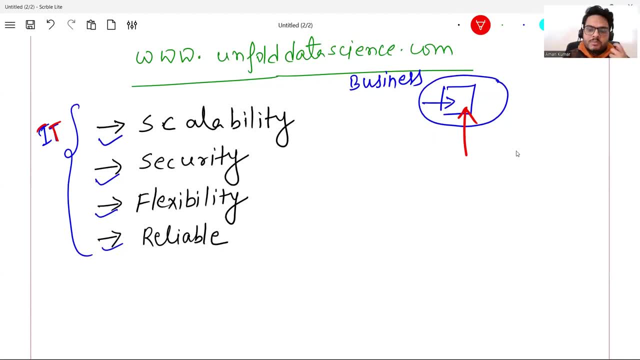 who are making shampoos, some famous hair care products, some big big pharma companies- right, they should focus more on their research, their business, how to grow market, how to do advertisement sector right, and less on how IT will be managed. that is where cloud computing, or all these cloud. 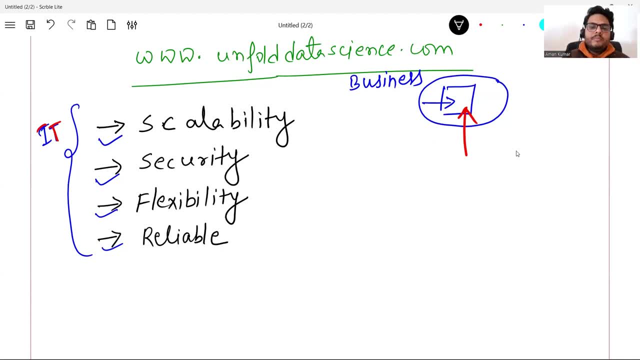 service provider comes into picture. what they say is: you give us money. I am writing here, you give us money, okay, I take care of your IT. I take care of your IT. this definition, guys. remember this and you will never confuse what is the meaning of cloud computing. okay, this is the basic. 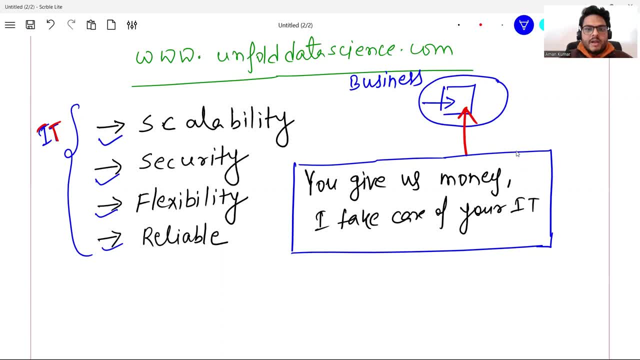 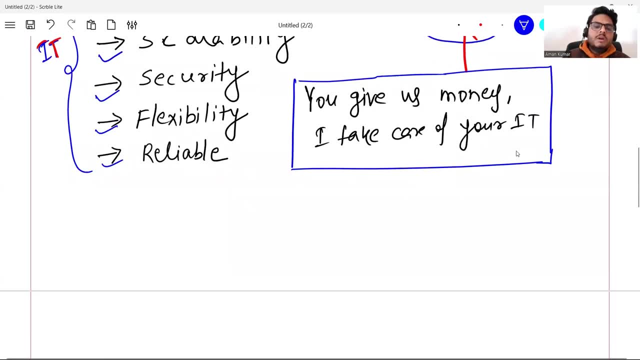 simple meaning. so I take my entire content, I take all my data, I host it on a cloud service provider. now I am using this word many times: cloud service provider. cloud service provider is an organization or entity that provides cloud computing services or that sells cloud computing services. okay, some of the big players in this space are AWS, standing for Amazon. 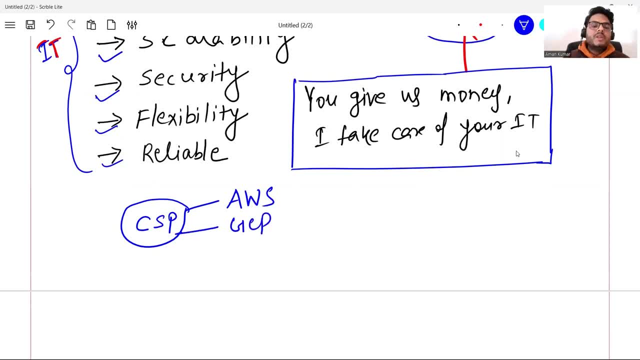 cloud services: GCP, Google Cloud Platform and Microsoft Azure. okay, why I am writing these three names is only these three capture almost 70 percent, 65 percent plus, that is for sure. I think it will be reaching 70 percent Now- of cloud computing market. okay, and why I am focusing on AWS in this series is AWS: 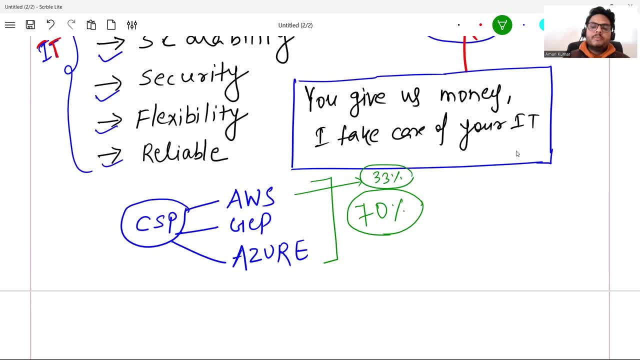 itself is roughly 33% of the total global market capture. okay, so one third of total global market of cloud computing is AWS itself cloud service provider as a service provider. okay, that is the reason we are learning AWS. so what is the simple definition of cloud guys? 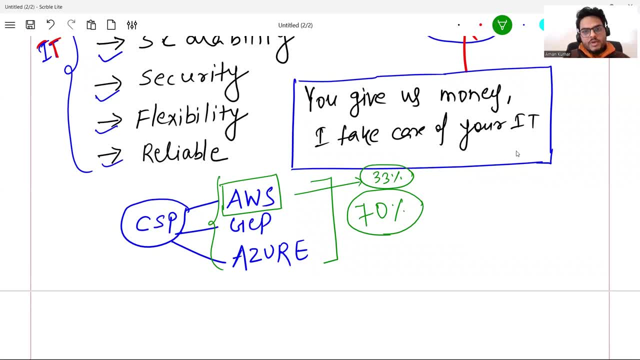 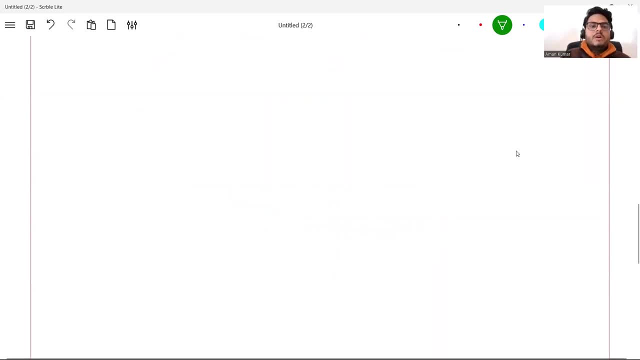 These service providers, you, you give us money and I take care of your IT. okay, what is the meaning of taking care of your IT, guys? one simple example I will give you. okay, let's say, in your computer you have a file. okay, this file, this one file, is your. let's say, let's say, daily workout schedule: okay, so daily you go. 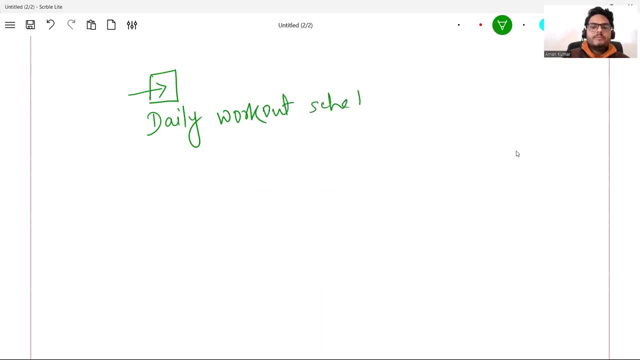 to gym and this is daily workout schedule- okay, schedule. and there is another file, I will call it. this is, let's say, file one. there is another file, file two. this is, you know what, this is your monthly expense, monthly expense calculator. okay, so first file, file one. you use how many times in? 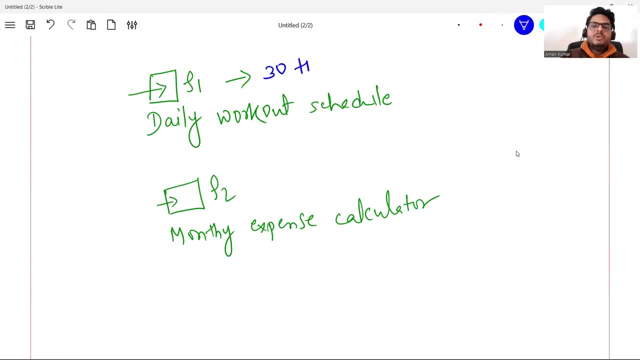 a month. you use 30 times in a month. I am thinking you go to gym daily 30 times in a month. you use this file and this file. you know how many times you use in a month? only once, okay, one time in a month, obviously, as a normal practice, what we do. we want to keep these kind of files on desktop so that we can. 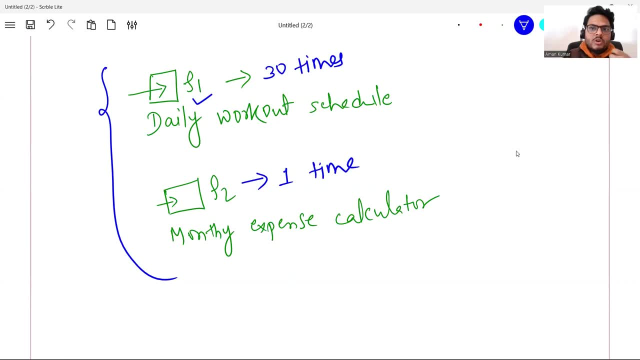 easily access it. okay, some files which we don't, you know, normally access, we keep it on some d drive, some inside folders, right, and we expect low latency here. what we expect: low latency. low latency means if I want to open this file, this file should open fast, right, I should be able to. 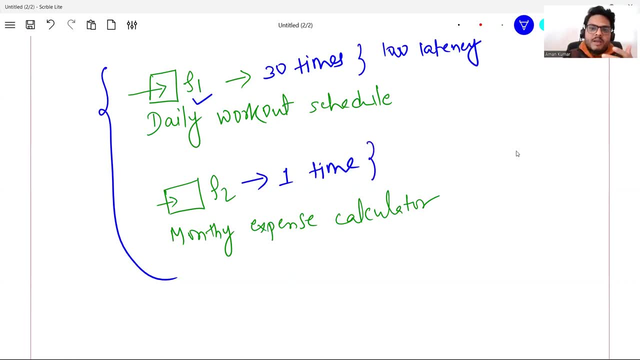 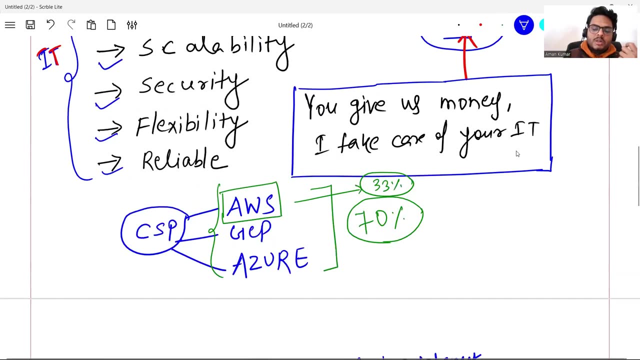 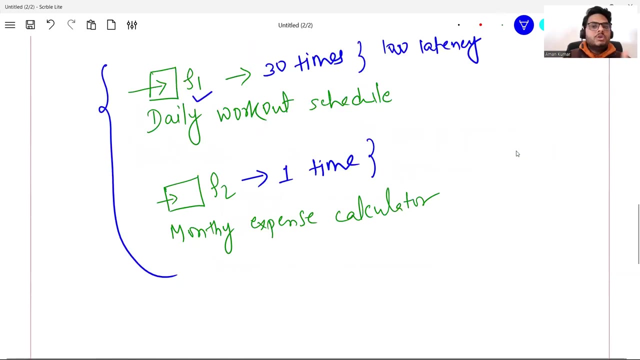 access this fast and this file, even if it takes some time. I don't bother because you know I do it monthly once. so in spite of doing you all these things, I mean this is just a part of what cloud computing can do. but what I'm trying to tell you is, in addition to normal things in your 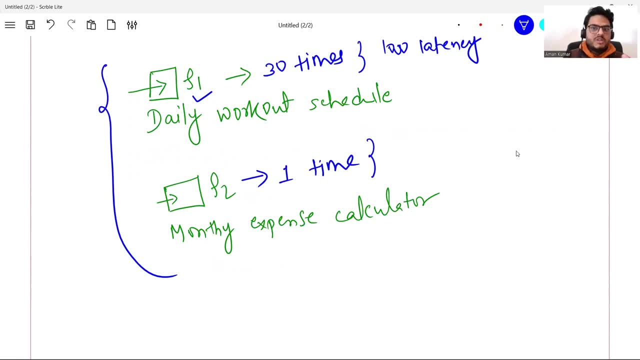 IT. it makes your IT infrastructure smart also, smart means cloud computing will enable you to have low latency on frequently accessed file and kind of little high latency on files which are less frequently accessed, of course, at the cost of money. they will charge you more for these kind of files, less for these kind of files. okay, we will see in. 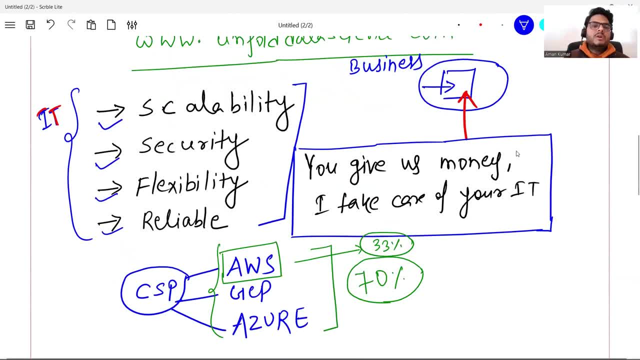 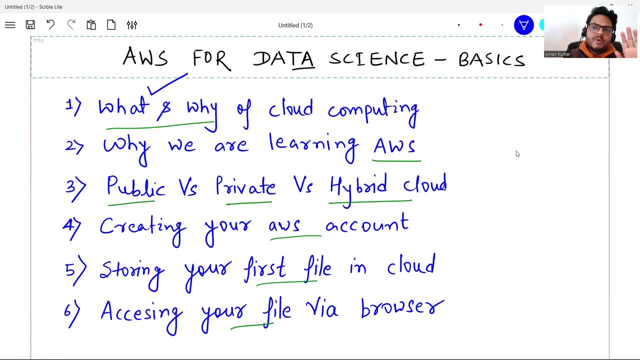 the demo now, don't worry. so these are some of the basics of cloud computing, guys, you need to understand. so what is cloud computing? I told you, for any business, if you want cloud computing provider to take care of your IT and that that becomes your clouding cloud, some service provider. 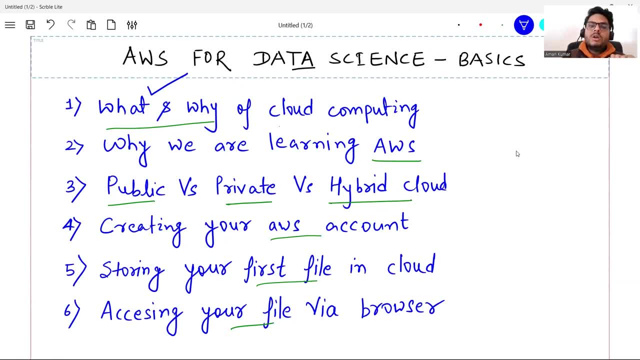 and entire thing that happens on their platform is called cloud computing. okay, and why cloud computing? because businesses want to focus on their core business, not on the IT side of it, and they want to, you know, utilize their bandwidth in focusing on business growth, not on the IT side of it, and that makes sense also. 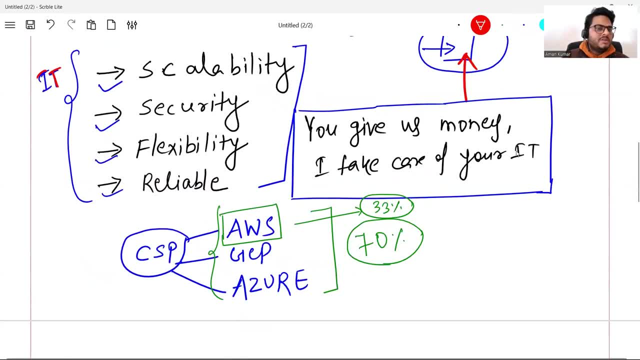 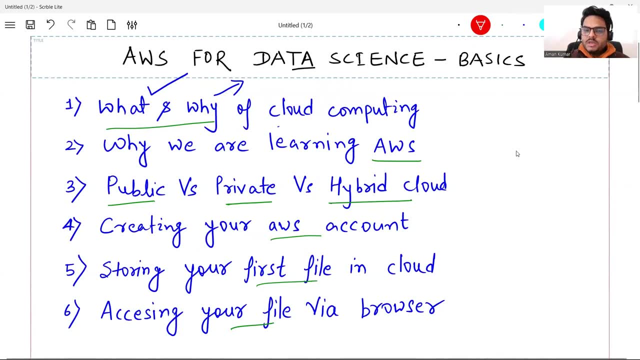 right, and why not? if somebody is giving all these things at a low cost, you know people will go and take it. okay, so we will see in due detail. but this is just a non-bookish to understand kind of definition. you can relate to unfold data science website and try to understand this. okay, why we. 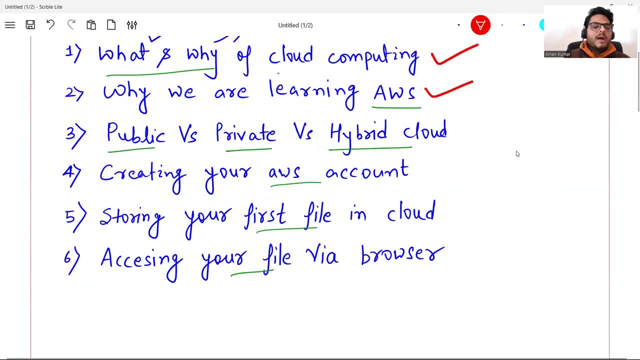 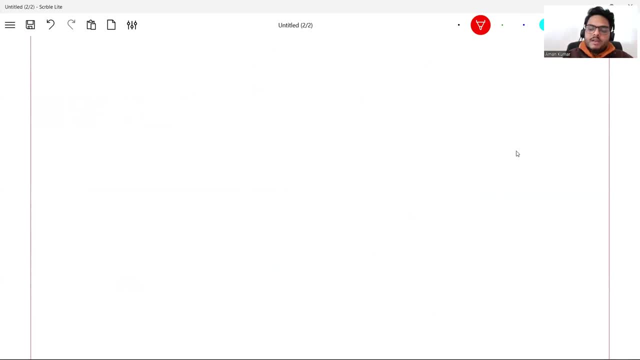 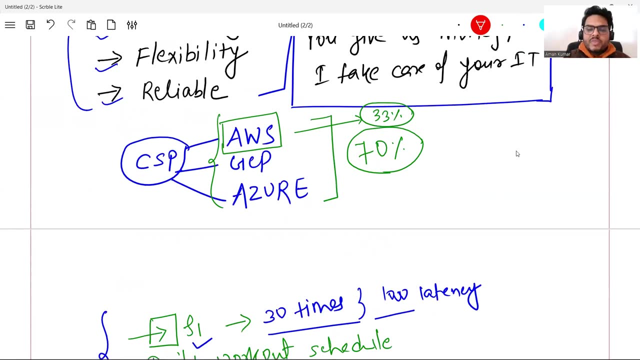 are learning AWS. I already told you. now I will tell you there are three different variants of, or three different kinds of services that cloud service provider can give you. okay, so who are cloud service provider? again, AWS, GCP and Azure, kind of guy. here we are talking about AWS in particular. now guys suppose in unfold data. 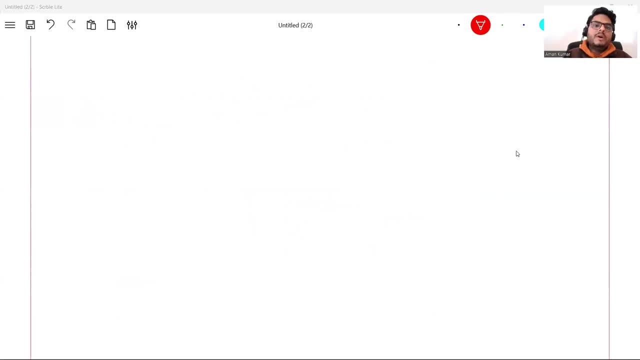 science website, what all things, from the IT point of view, I need to take care? okay, suppose in unfold data science website, from IT point of view, what are the things I need to take care? I will just keep writing here, okay, so that I'll tell you what is the difference between three types of services that we take from cloud. 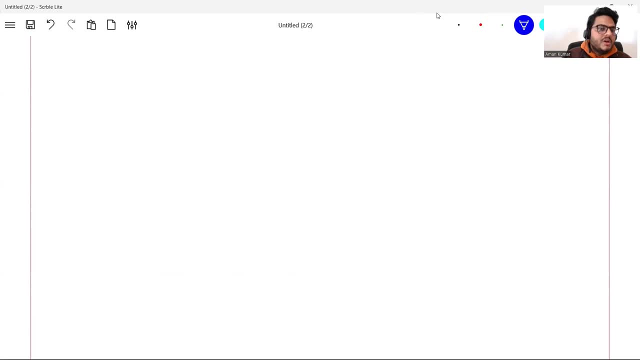 with example, not by bookish definition. okay, first of all, I should have application. application means I am hosting my courses right, so courses should be there, quizzes should be there, assignments should be there, so that is part of my application. okay, then comes my data. data is nothing but. 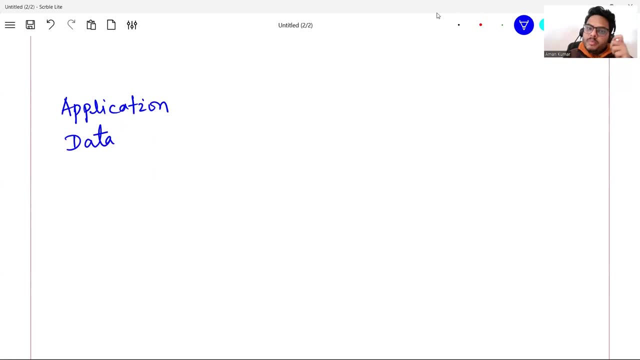 user data, my, you know, maintenance of my users or addition of new user or deletion of user or what. what file formats I'm using, what files I'm adding right application data- I'm just looking at my notebook so that I should not miss any anything. runtime: the meaning of runtime is when my 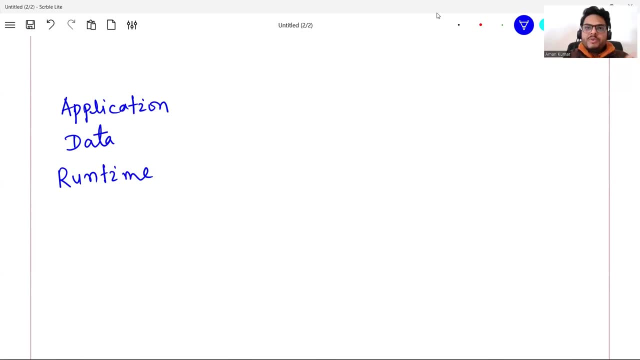 application runs, then it should be managed in a proper way so that front-end users are not facing any issues. okay, then comes middleware. middleware means: is it calling to some apis, or is it? is it doing some kind of communication with the back end? right, that part will come into picture. and then comes the operating system where it is. 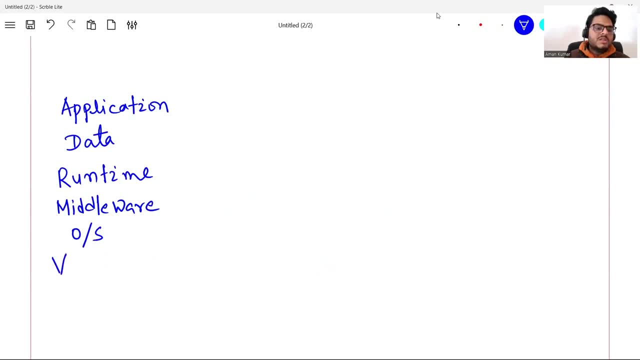 running, on which os it is running. and then comes virtualization, if any. it is not always needed, but if any virtualization is happening, which means if it is running on any vm or any virtual servers, then that will come into picture. and then comes: what servers is getting? 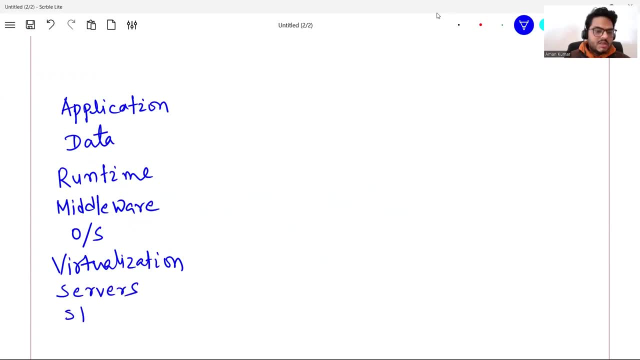 used- okay. and then comes what storage is getting used- okay. and then comes what networking is getting used- network, okay. now I will write here three terms, guys. I'm sure you have heard about this. one is called infrastructure as a service- okay, I A A S. one is called platform as a service- P A A S. and one. 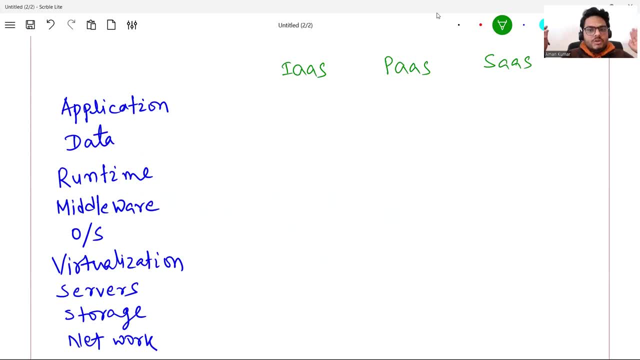 is called software as a service. okay, don't forget all the definitions that you know about all these things. okay, again relate to unfold data science. so what all should be taken care when a course hosted on unfold data science website is accessed by a student? okay, application data runtime middleware- all these may not be. 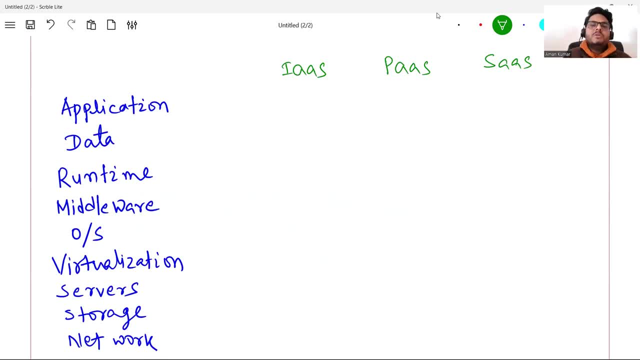 applicable for all the applications. for example, let's say I'm hosting on a local machine and from local only I'm accessing, so virtualization will not come into picture. I'm not using any VM. okay. similarly, I'm using, you know, storage, local storage. so storage is not very complex in. 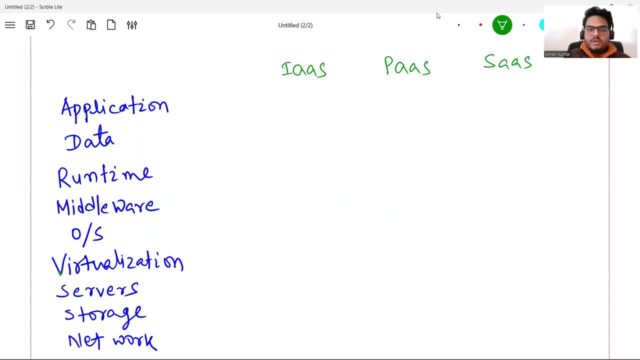 that case. but overall, all these things will come into picture if I am running a full-fledged application. okay, remember what I'm going to tell you now. this is an interview question. people will ask you: suppose aman does not use any cloud services. suppose aman does not use any cloud. 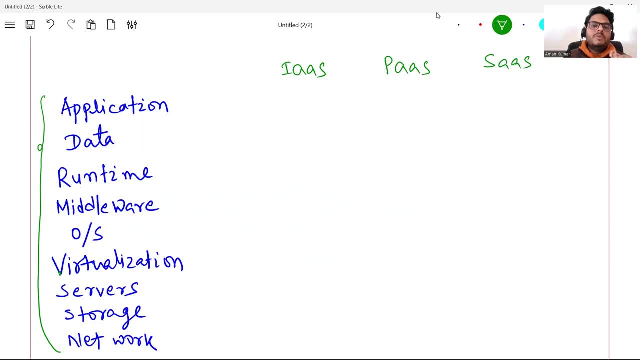 services and maintains, runs the website, the platform, by himself. so what all things aman is responsible for? aman is responsible for everything from here to here. okay, everything from here to here. aman is responsible because aman is not outsourcing kind of his ID, aman is not using any cloud service, aman is. 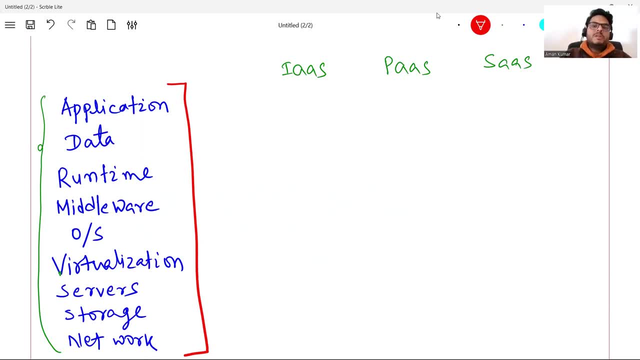 responsible for all these things. okay, take a moment, guys, try to understand. now suppose aman aman's business grows and aman wants to, you know, give some part of it to a cloud service provider. so aman decides that I will take care of from applications till OS. okay, 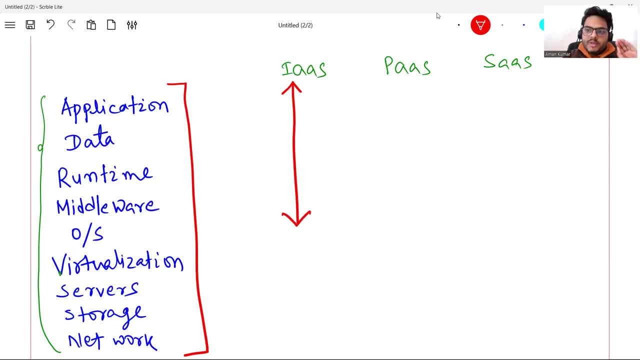 from applications till OS. I will take care of my application, I will take care of my data, I will take care of my runtime, middleware and OS, but but I want the cloud service provider to give me virtualization. if any, I will use your servers, I will use your storage, I will use your network. 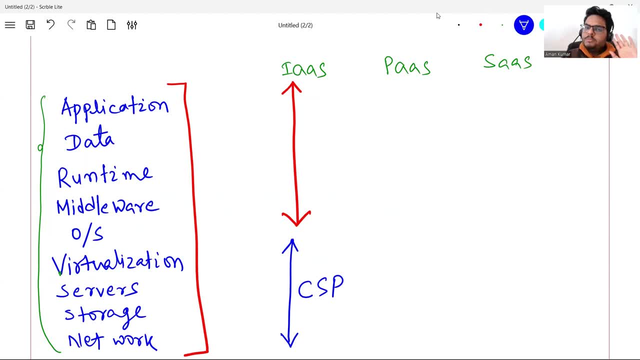 this becomes infrastructure as a service- simple definition, okay, from the cloud platform, what you are taking, what you are renting, is infrastructure. what infrastructure you are renting? virtualization is storage and network capabilities of the cloud service provider. fine, when we see the AWS console, I will show you what all comes under these categories, don't worry. okay, so infrastructure. 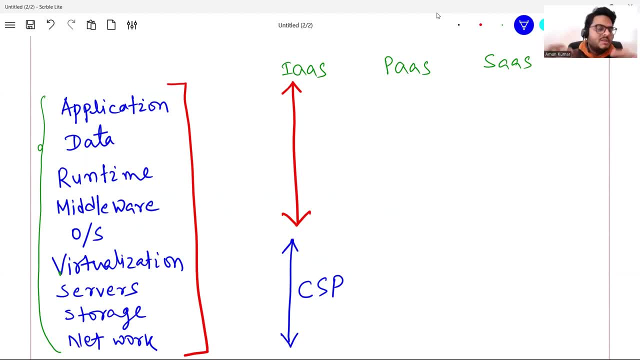 as a service is basically you give me the infra, rest of the things I will take care. so you give me the storage, you give me the server, rest of the things, I will take care. so that is kind of least use of cloud platform you can say, and mostly the company or the enterprise or the business itself is: 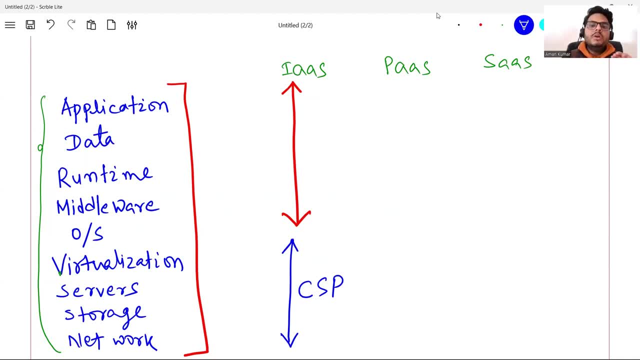 most of the things. this becomes your IAS standing for infrastructure as a service. now, what happens in platform as a service? in platform as a service, everything right from run, runtime, everything right from runtime till end will be managed by cloud service provider. okay, so what you are managing? 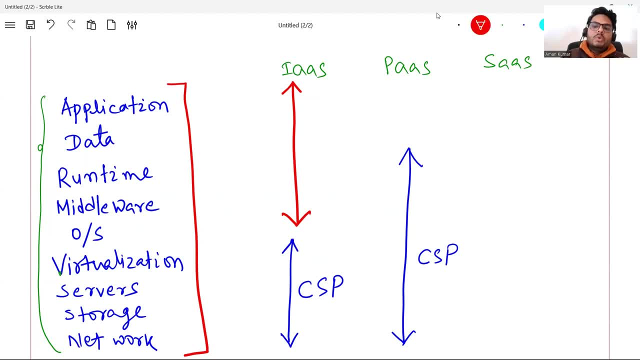 you are just managing your application and data. what you are managing, you are just managing your application and data. so, if you want to add a new feature in the application, if you want to, as a you know, delete a feature from your application, if you want to do something with your data, those 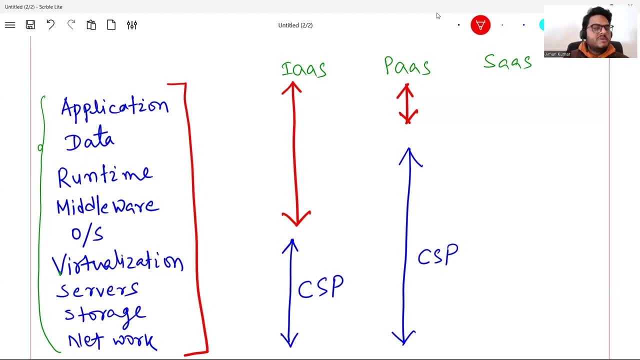 things you manage. apart from that, everything is managed by cloud service provider. that is the definition of platform as a service. I will give you examples in all these three categories. okay, and then comes software as a service. what happens in software as a service? everything is managed by cloud service provider. you just use that software. okay, everything happens on cloud you. 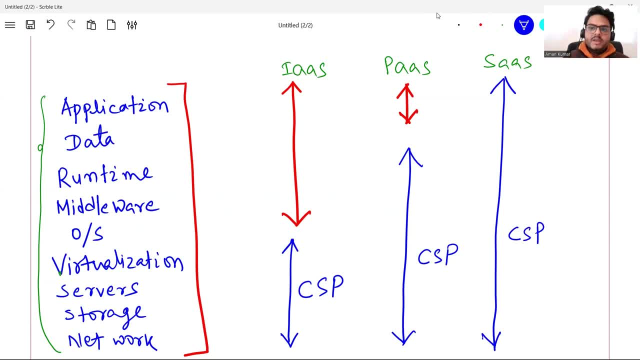 just use the software as an end user. examples in software as a service category. here are some examples I have noted. guys, you must be using something known as Dropbox. I am sure you have heard this. sorry Dropbox. Dropbox is nothing but a cloud, uh storage given to you where you can store, file retrieve later. so what you are doing here, you are just using. 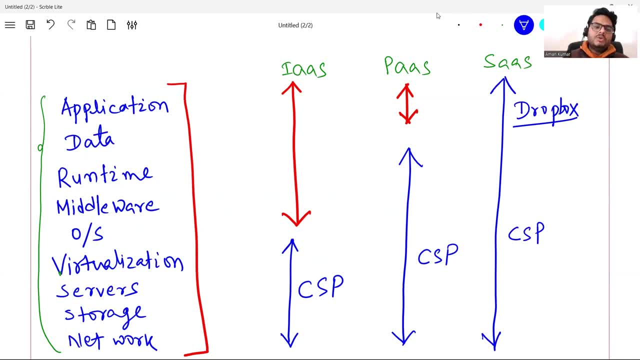 software as a service. you are not managing application. nothing you are doing. you are just as an end user. you are using Dropbox to store your files. very simple. Microsoft 365, okay. your Excel, your PowerPoint, your word, all these things, what you are doing. you are using those. 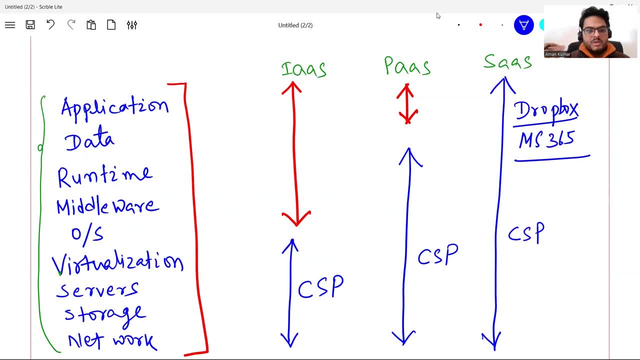 applications. you don't bother about how the runtime is, how the middleware is, how the virtualization is, how the server is, storage is, if you are in a you know- um aws, sorry, azure cloud kind of platform. okay, then one more example i will give you, which most of you would have used: cisco webex. okay, cisco webex in cisco. 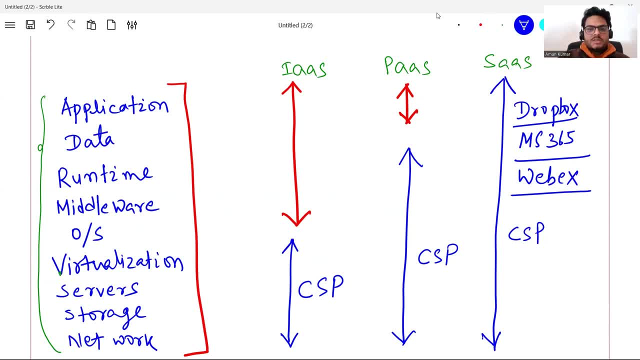 webex. what you use, you use just the front end, just the application. you don't care what is the software code written, what is the storage written? uh, how much data i will be storing where it will get stored? you just do the meeting, your file gets stored. later you can, you know, get that file. 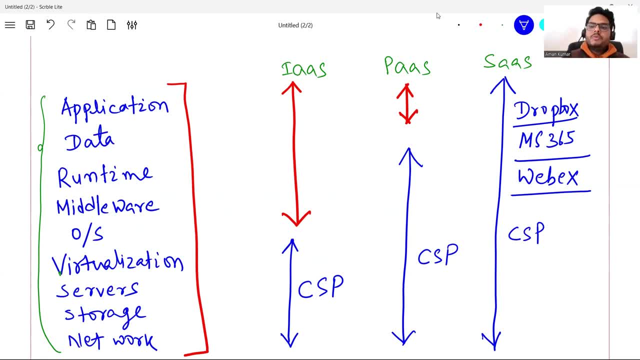 that's all, end of the story. all these are example of software as a service, where you are an end user. okay, now suppose you are not an end user, you are a team of developers. so here you are managing some bit of it. some bit of it. you are managing your application. you are managing your. 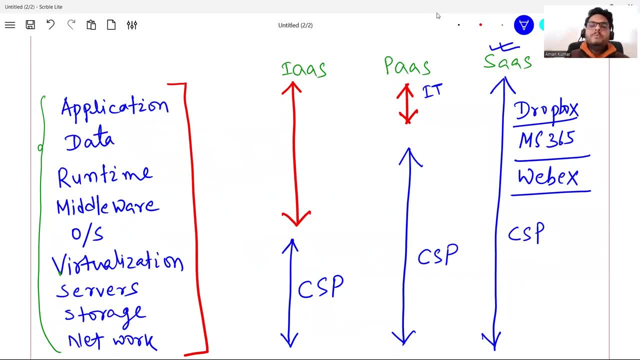 data you are managing. you just say to cloud guys: hey, give me your platform. okay, i want to host you my application on your platform. give me your platform, that's all. okay, that's all i need. i have the expertise to manage my application and data those guys will. 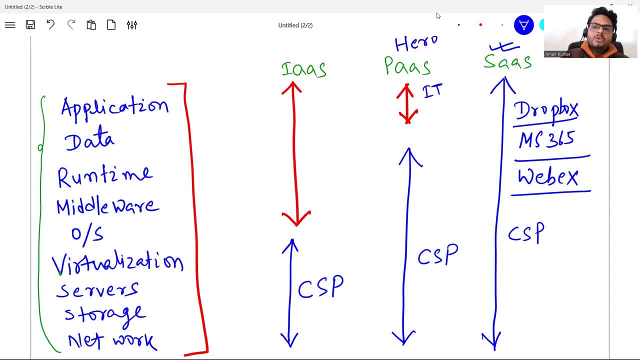 give you, and one kind of example here will be heroku. if some of you have hosted your application on heroku- you know data science application or any kind of web app- you will see that you are managing your code, you are managing your data. you are managing code means you are managing your. 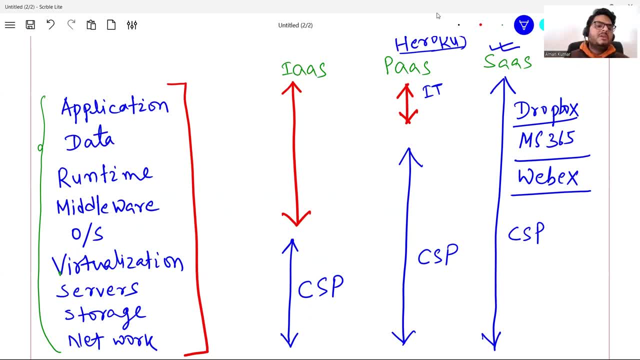 application cloud service provider is giving you everything right, from runtime to virtualization, to middleware, everything okay. so this is, you know, middle, middle level it expertise. okay, middle level it expertise. this is zero. itx software as a service. zero it expertise platform as a service- middle level it. 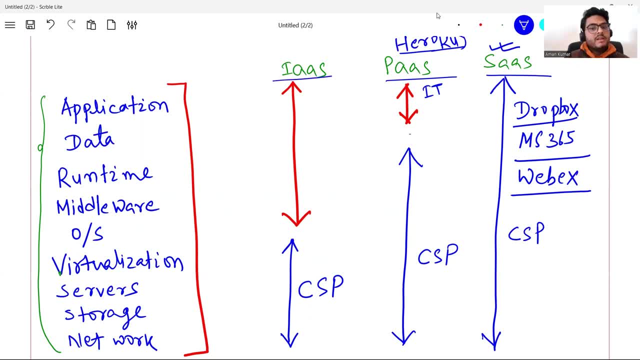 expertise, and infrastructure as a service means more it expertise. you are saying, hey, just give me the infra, i will take care of rest of the things. okay, here, you will just take the infra and you can do whatever you want. so many kind of application which are hosted on the cloud and being managed by um individual organizations. okay, that can come. 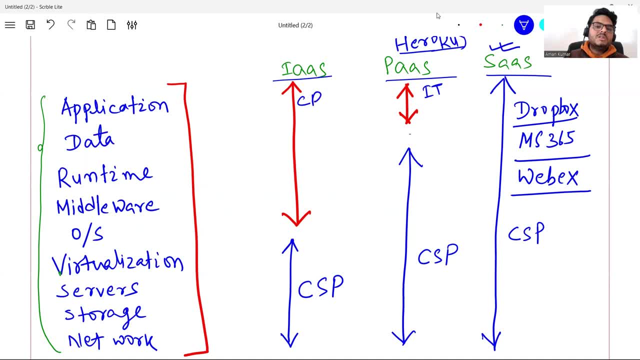 under infrastructure service. for example, some of the crm applications organizations host on the cloud. some of the invoicing applications some organization host on the cloud. they want to keep the data secure and they want to have most of the control, apart from just they are renting the apartment. you can say, for example, you rent a apartment to stay. 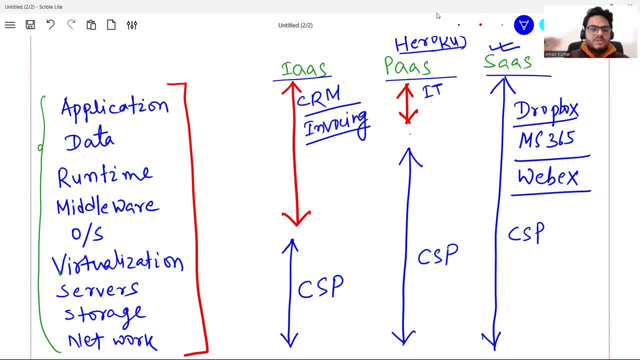 whatever you do in the apartment, that's your business, right? you rent the servers, you rent the storage, then you do whatever you mean. so anybody asks you the difference between ies, pas sas. remember the difference: sas list control. all the control is with cloud service provider. 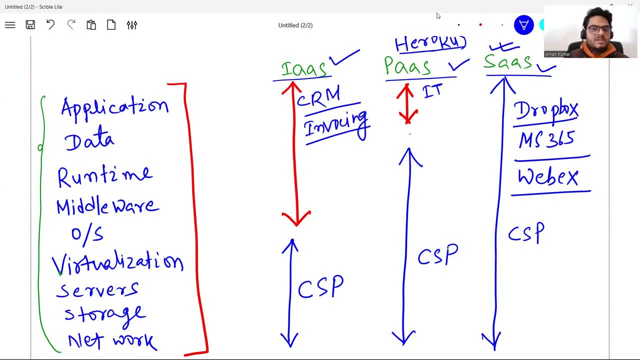 ps. middle level control is more control. these are the things that will be controlled by cloud service provider in all these categories. okay, so this is basic of three different types of services that cloud computing provider, cloud service provider will provide you. in all these categories you will see different, different. 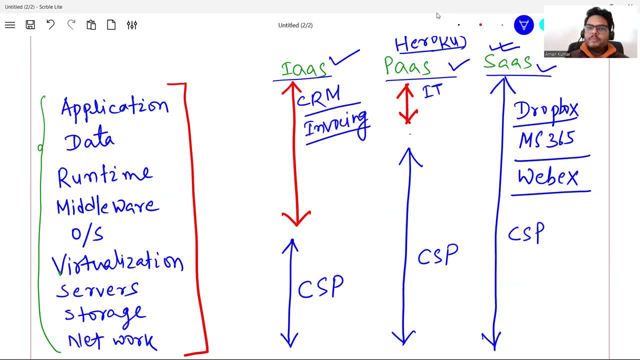 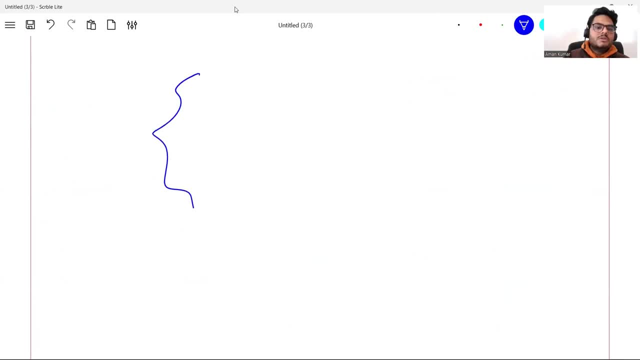 components. we will show you in aws. i will show you in aws console. okay, now one simple and straightforward concept i want to cover here. guys, uh, suppose this is your cloud? okay, uh, cloud service provider or you know cloud, you can say: and this is your other cloud, okay, so there is a terminology called public cloud. okay, one simple concept here. 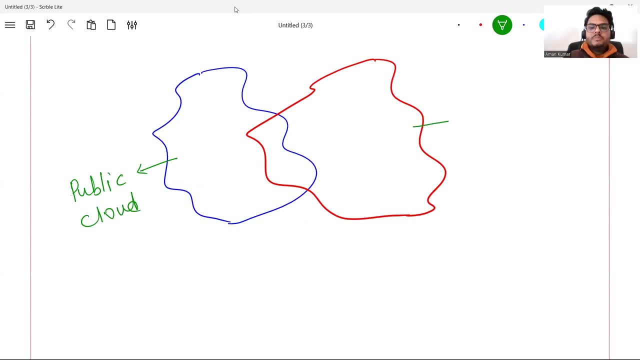 public cloud and there is a concept called private cloud- okay, private cloud. and there is a concept of hybrid cloud- hybrid cloud- okay. so, guys, you have to understand what is the difference between public cloud, private cloud and hybrid cloud. suppose i'm i want to host and for data science website on aws. okay, so i will. i don't care much about my data security. 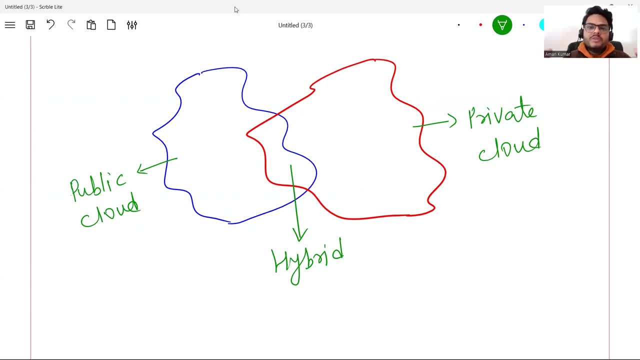 because it's it's like you know, students name and email and it's not very, very sensitive data. okay, students name and email id and my my course files, right. so what i will do is i will look for a little cheaper option to host in aws, and the cheapest option is using public cloud. okay, public cloud. 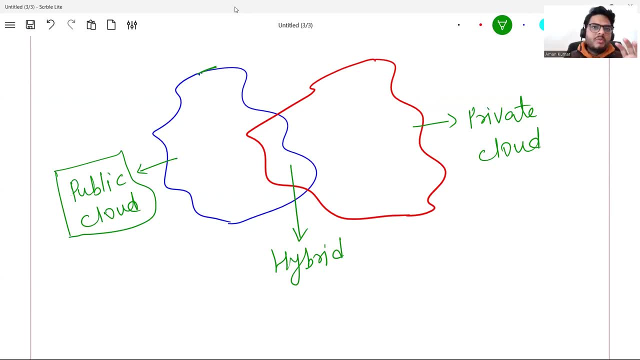 means wherever you are hosting your application. you can use public cloud to host your application or wherever in the in the cloud the cloud service provider is allowing you to host it in a public space where somebody else can also host their application. it will be secure, of course, by 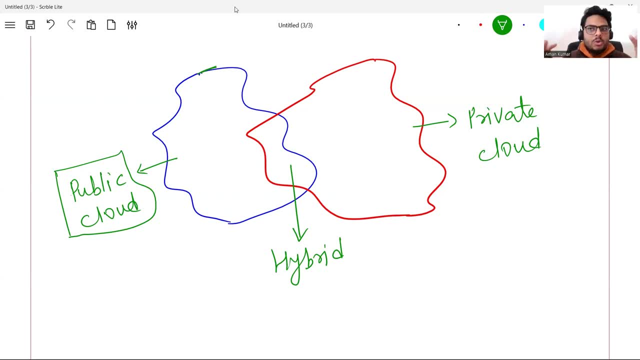 multiple security protocols, but in public cloud, many, many customers of the cloud service provider can use the application to keep it very simple. okay, but think of a scenario where it's a bank- okay, it's a bank in the bank. the data is very, very sensitive. customers, account balance, card number, pin, you know, debit card pin. 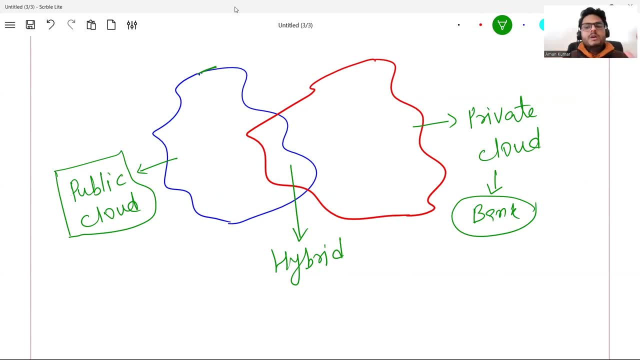 or cvv number, etc. so banks will not want to use the public cloud because, by mistake, if something happens, okay, then their data may get. they are afraid that, though the cloud service provider say that your data will not get exposed, but they are afraid that it may get exposed and also 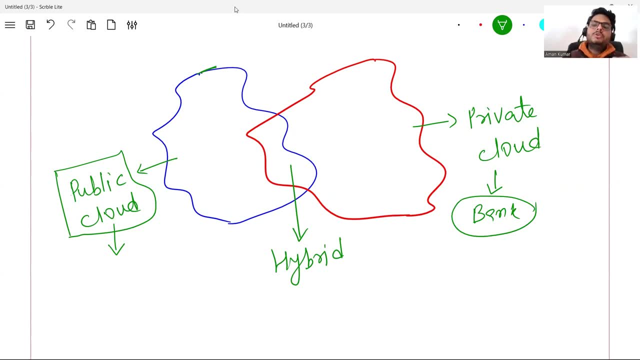 there are a lot of security protocols they need to follow on their data. so if you want to store something sensitive on the cloud, okay, remember this. if you want to store something sensitive, which which is very, very sensitive and very, very private, then you will use private cloud. if you want to, you know, store or use cloud service provider for normal things, not too. 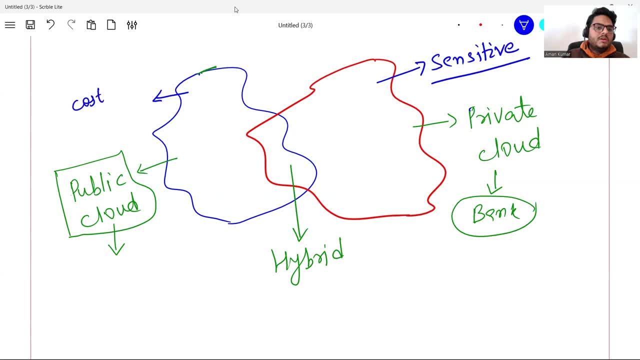 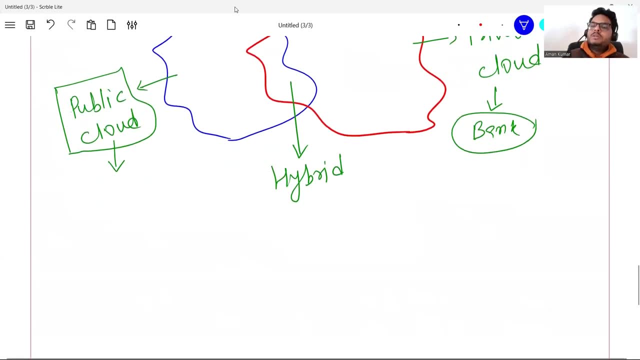 sensitive, you will use a cost effective method or cost effective flavor. that is known as public cloud. in any organization, it will be a mix of both. so they go for hybrid cloud. why? there are three different concepts, guys. in terms of dollar, you know, charge that cloud service provider will pay. 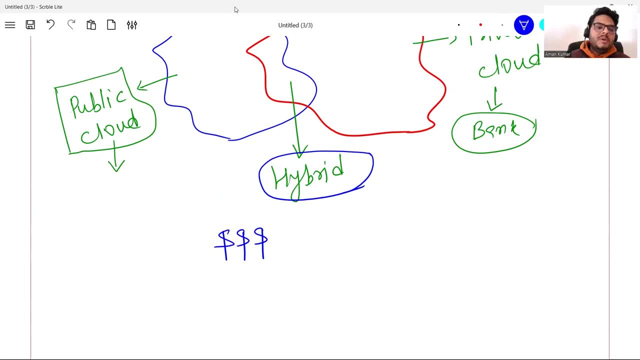 you know, charge you for the service, right, it will be leased in public cloud, it will be highest in private cloud and it will be somewhere mid-level in hybrid cloud. okay, but sometimes if you want to store sensitive data or banks do not want to compromise, they will go for private cloud. 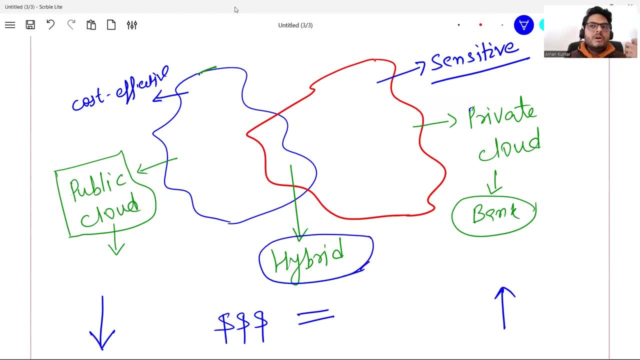 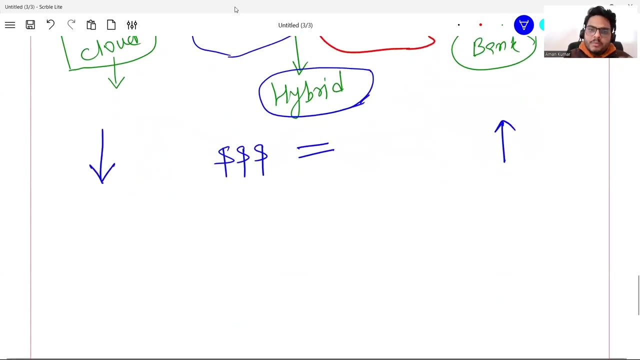 otherwise hybrid cloud and public cloud for good for the businesses where we want a cost effective solution. we are a small business and we don't want, you know, not not lot of security protocols we have to follow on the data sector, just an example i give you. now there are more. 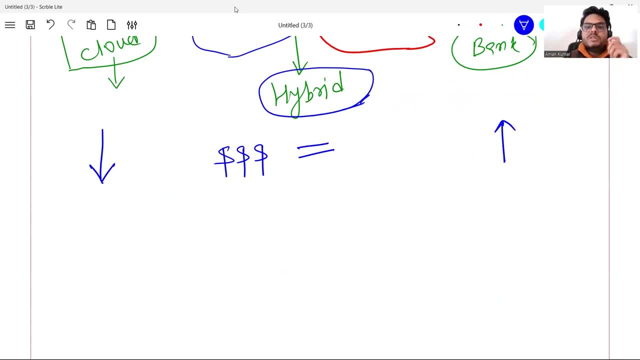 differences to this. for example, if you, if you say who is the owner of a private cloud, so here company itself will be the owner of this cloud. okay, in terms of owner. i'm saying owner is company. okay, who is the owner of a public cloud? owner is cloud service provider. 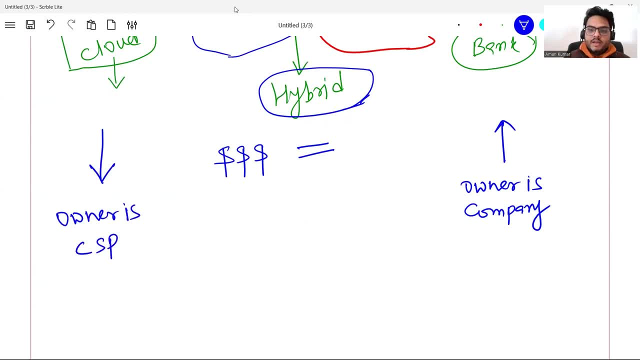 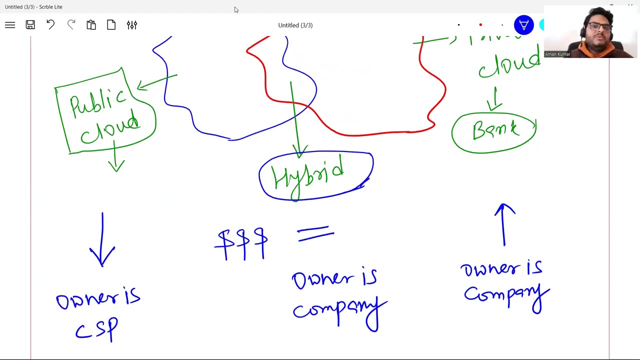 owner is cloud service provider: okay, and in the hybrid cloud also, owner is company. company means if unfold data science, then unfold data science is the owner of this. okay, so you can compare public, hybrid and private cloud in terms of uh many things. for example, if you ask me where the 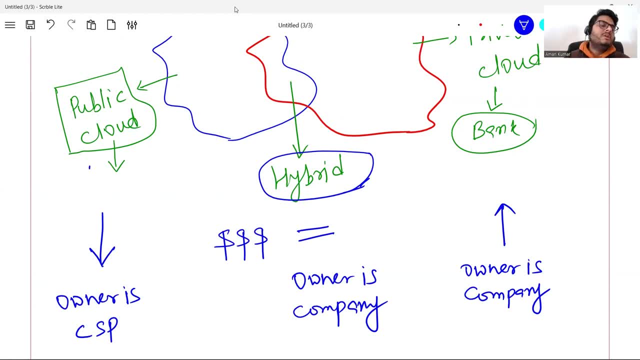 scalability and flexibility will be more obviously. in public cloud it will be more because private cloud there will be again a lot of restrictions coming, a lot of protocols coming right. if you ask me where the charges will be? less, of course, public cloud. if you ask me who. 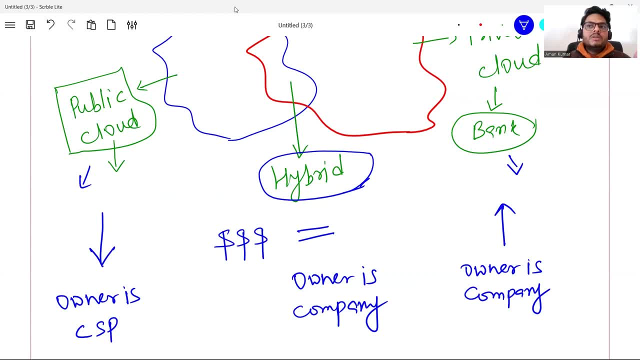 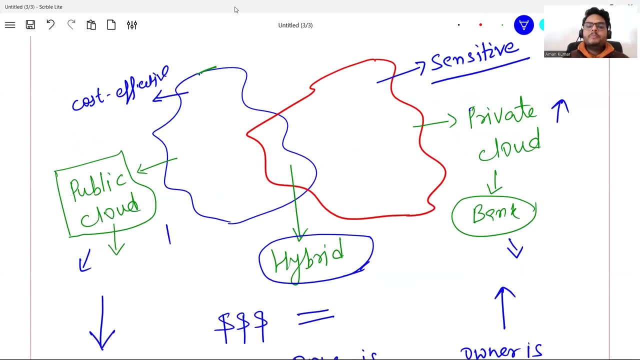 will own, this guy will own. if you ask me what is the reliability and what is the security, obviously hybrid cloud will have more security. private cloud will have more security than public cloud. okay, so somebody asks you the difference. you have a overall idea. i will not explain you more. i don't. 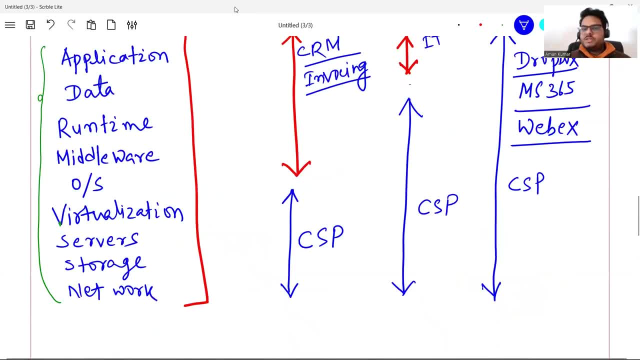 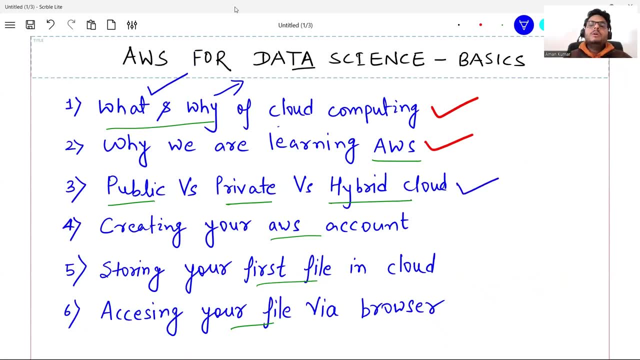 want to confuse you. i want to go to the lab first. okay, now what we learned, guys. we learned public private hybrid cloud. i also explained you how do you, uh, differentiate between infrastructure as a service platform and software as a service. now it's high time let's go and do some lab, guys. um, let's create your first. this is called aws. 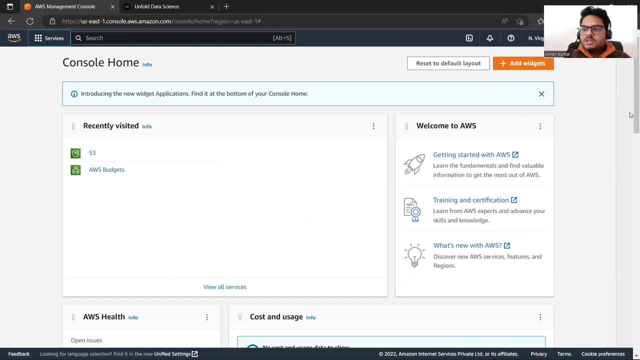 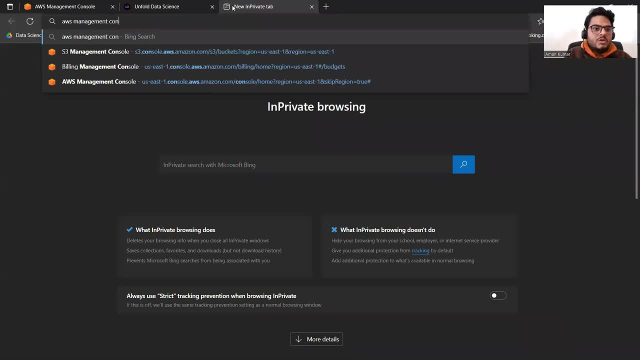 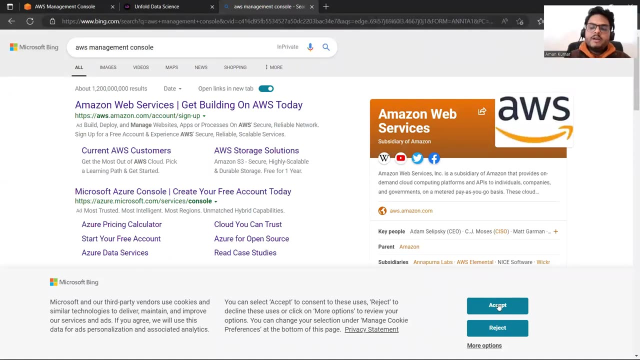 management console. okay, and i am logged into this, but what you can do is you can go to google and search for aws management console. aws stands for amazon website web service, one of the leading cloud service provider, and my entire playlist, or my entire series, will depend on aws itself. okay, so if i go to aws, 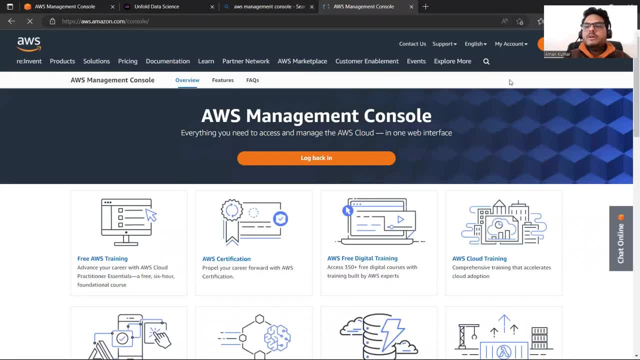 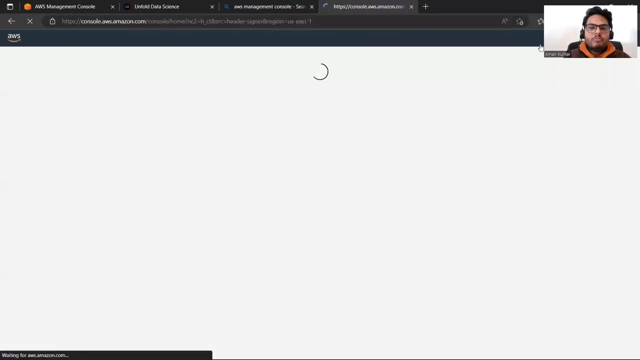 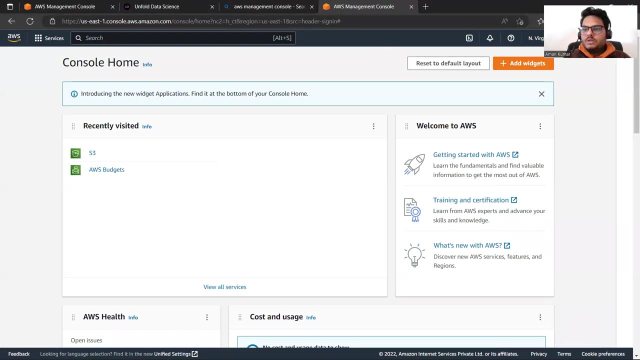 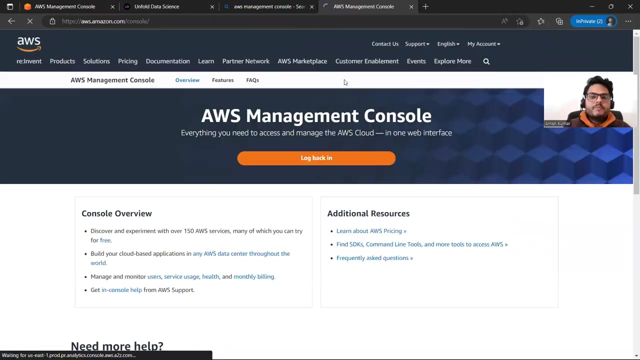 management console. here then what you can do. guys, you can see a button here to create a new account, okay, so here you will click on this. i think i'm logged in, so it is taking to my account. let me log out first. give me a moment, let me log out. okay. so this is my sign in to console, okay. 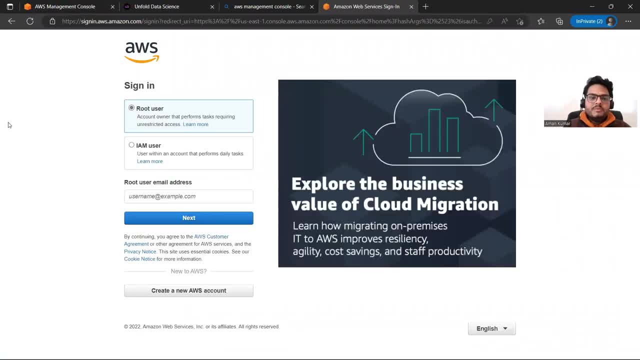 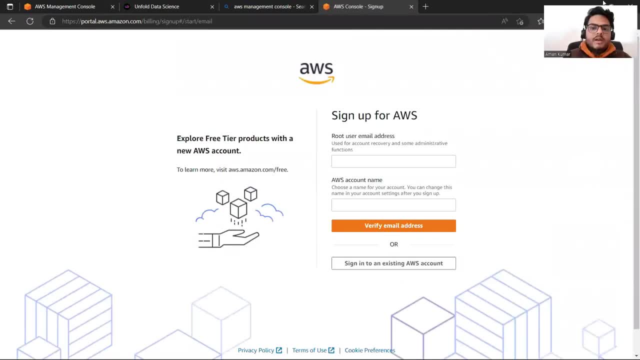 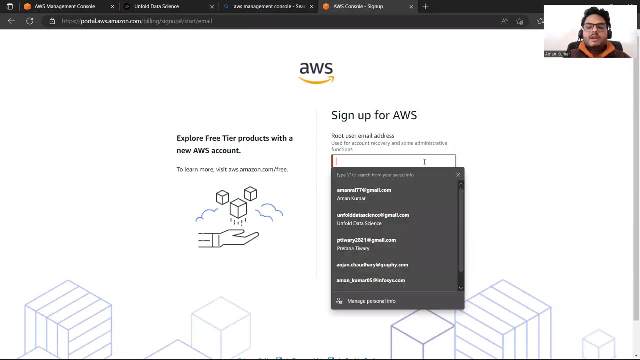 and is it remembering my password? no, it is not remembering my password. so first you have to do, guys what? create a new aws account. if you don't have an account, okay, and here first thing they will ask you is create your aws account with an email id. give an email id here. give an email id here. they will send you a passcode. 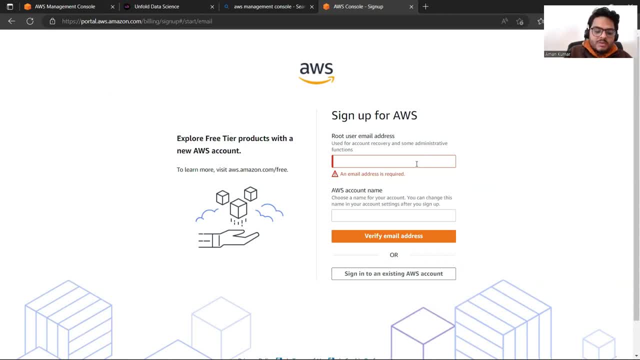 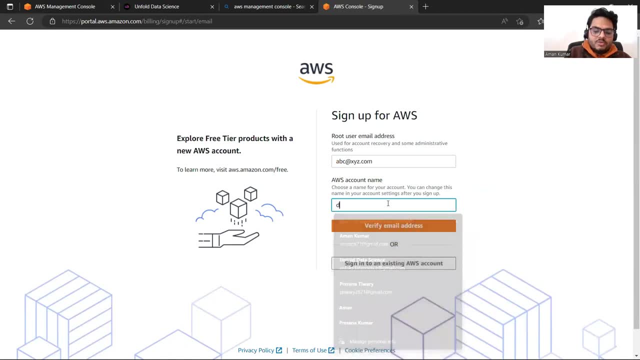 okay, that passcode you enter here. give a email id, for example abc. abc at xyzcom. okay, and you enter your name, so for example dummy name, okay, and then you say: verify email address. if you say they will send you a passcode, enter that passcode here and it will take you to the next step. next step: they: 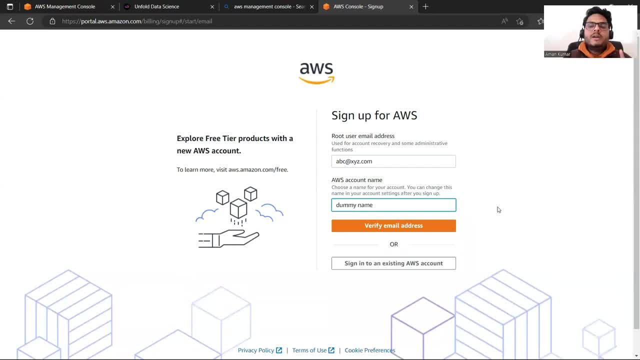 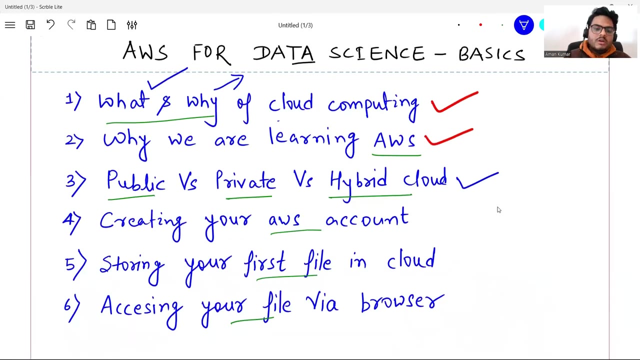 will ask you your name, address and credit card or debit card number. now remember, guys, without credit card or avatar, your account may not get created. so when i added my credit card- indian credit card- just two rupees i think got debited. okay, just two rupees. so don't be afraid, guys, you can add. 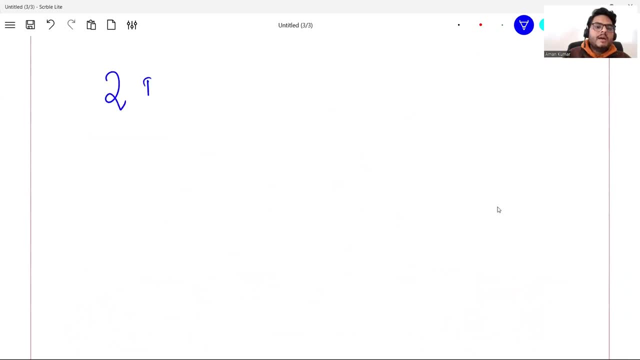 your credit card or debit card. just two rupees to inr. okay, two rupees will get deducted from your card. just two rupees will get deducted from your card, so you don't have to worry about having a to ensure that you are adding a valid card. okay, do that until or unless you use some heavy service. 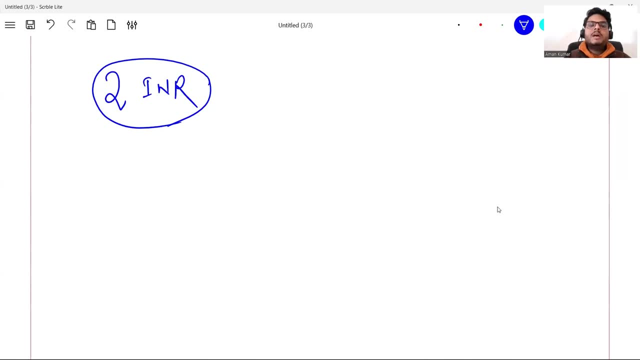 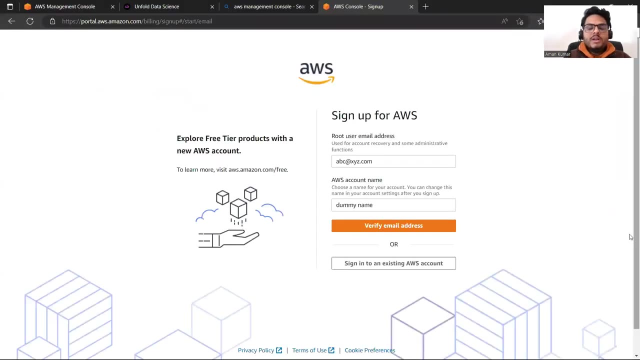 amazon will not charge, you don't be afraid. you can add that. i will also show you how you can control your budget. okay, so once you do that, then you are good. it's like normal um any any kind of account creation, okay, and then you have your user id and password created as a root, because you will 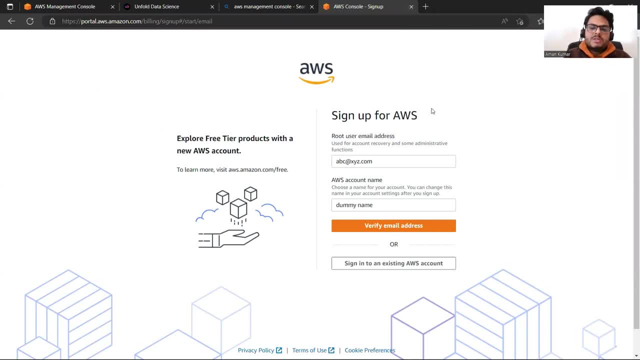 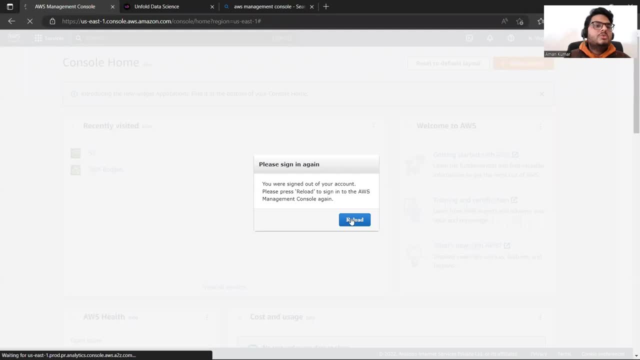 be on a root user email address you give, which means you are the master of that account. you are the owner of that account. okay, using root, you can create. once you create, you will come to something known as aws management console. so i am a root user. i have created my account. this is my user. 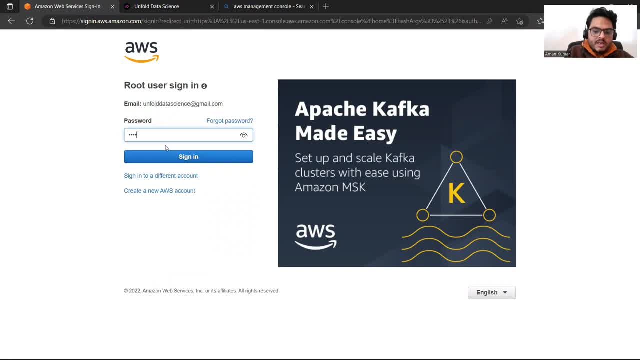 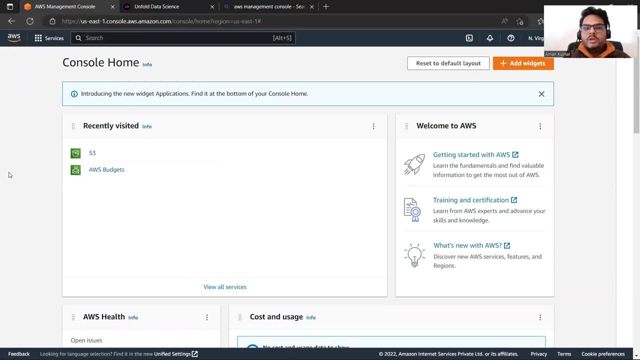 id password. i have saved it. let me try logging in. it is asking me again. let me try. okay, so i'm inside aws management console, which means amazon web service management console. if you are doing with me, congratulations, you are inside the first cloud service provider, aws. okay, now i told you. 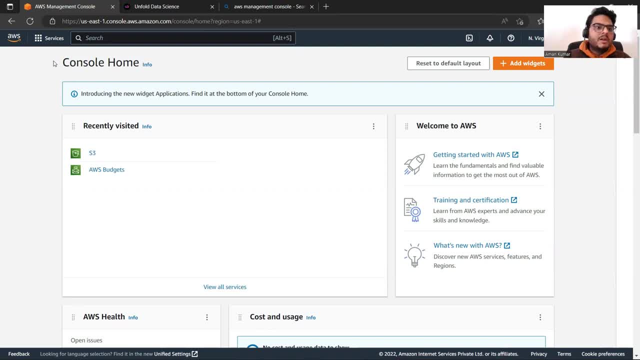 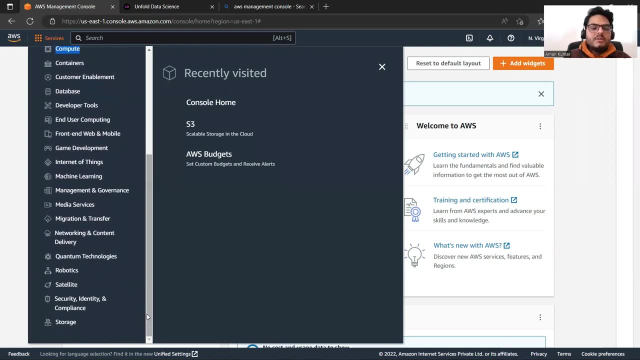 there are a lot of services that cloud you know service provider will provide. let's see what are the services. so, for example, i told you in storage, in storage, they will provide you different kind of services. so see, for example, i am in storage. okay, so here aws. 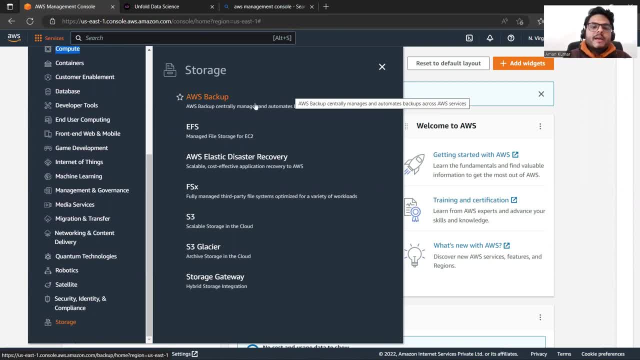 backup is one category of stories. okay, aws, elastic disaster recovery is another category of stories. okay, so in one liner they are trying to tell what is the use of these stories. so scalable, cost effective application recovery: okay, s3 is scalable. storage in cloud: simple one. s3- glacier is archive. 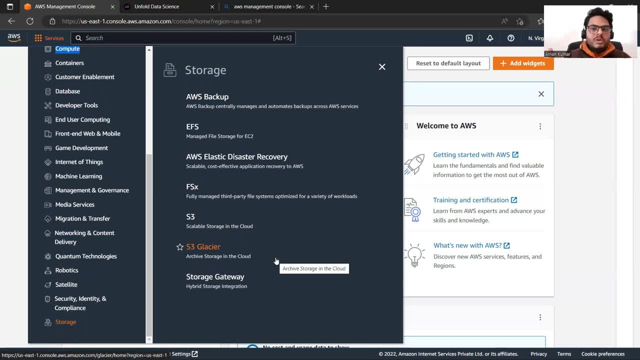 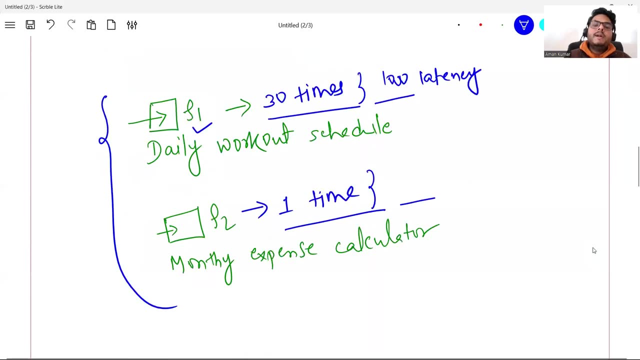 storage in the cloud. in my next session i will cover in more detail different stories and what are the functionalities provided in different stories. for now, just you remember i gave you one example, guys. you remember i gave you one example of file being used regularly and not being used regularly. so amazon web service enables you to become 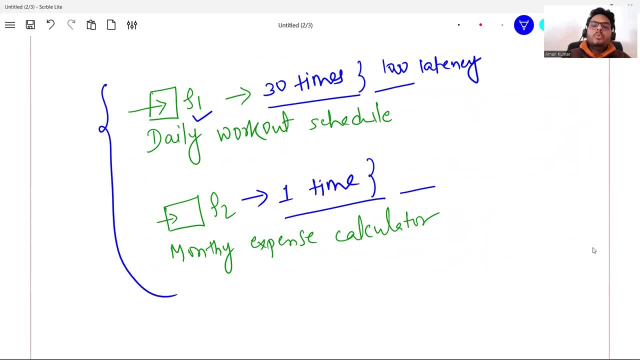 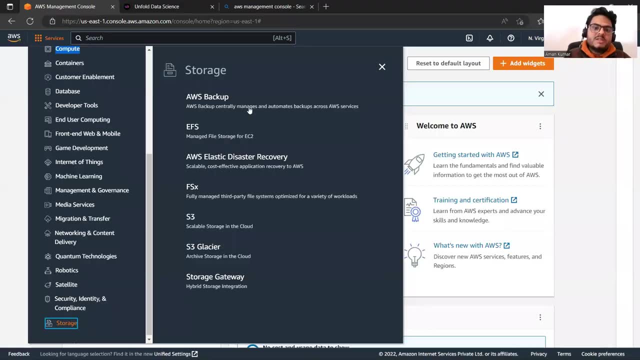 smart and save cost based on what is the, how many times you want to use that file, okay. and if you see multiple types of stories, all these is trying to serve one or other kind of service to you. for example, if you say glacier, glacier is one kind of archive, okay, so it will. 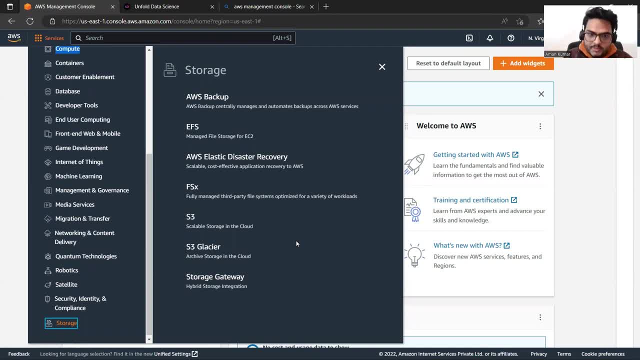 not be. it will not focus on low latency, it will focus on low cost. okay, and then managed file storage, efs, volume efs is applicable for something which you need many times and there are different purposes of different files. okay, what we are going to do is we are going to go to s3, which 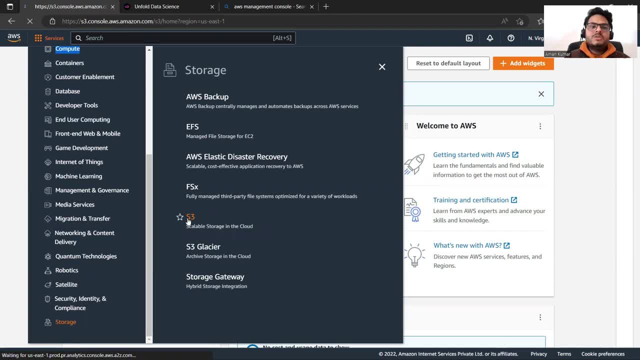 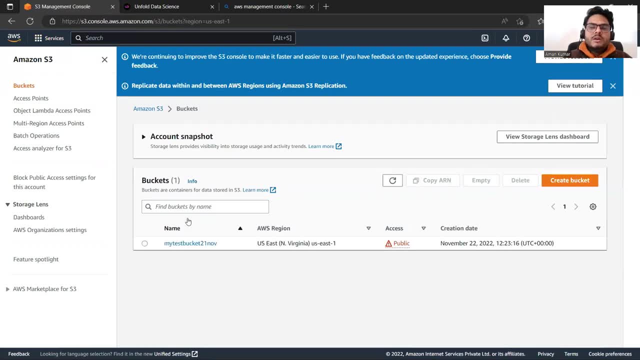 is known as scalable storage in the cloud. okay, let's open this s3. all of you can open this s3 is basically your. you can say, um, one root storage, uh, you know one kind of storage, simple storage service in cloud. okay, so let's come here and i want to explain you, if you want to. 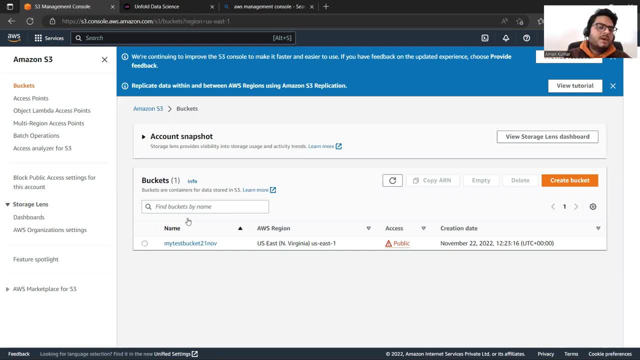 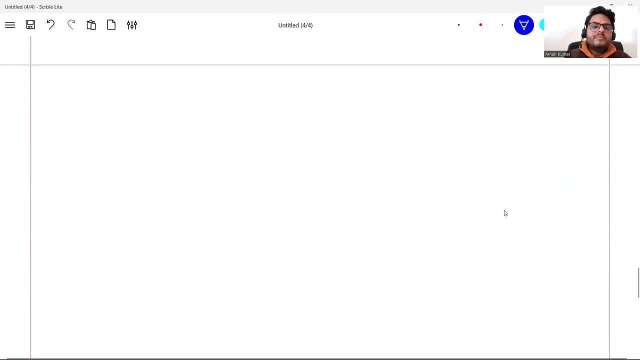 what? what we are going to do now is we are going to upload one file in the cloud, okay, and i want to tell you something here, guys, from theory, then you, uh, we will create that. okay, let's go to s3. what happens is in s3, there are two concepts, okay. one is called a bucket. 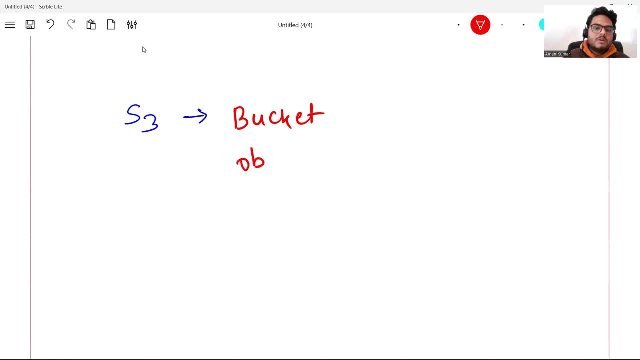 bucket and another is called a object. okay, what is a bucket, guys? a bucket is a common repository kind of thing. okay, so this is a common repository. inside one bucket you can have multiple objects. multiple objects means multiple files you can upload, no matter what is your format- video or 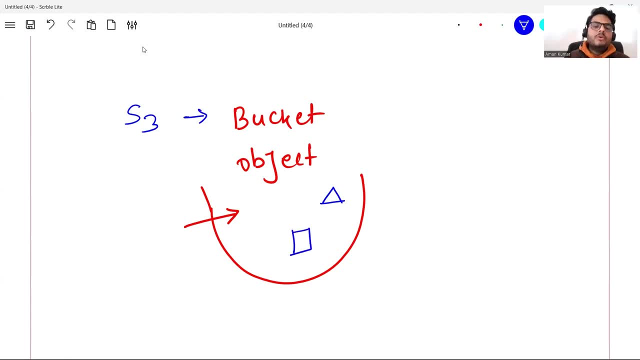 zip file, etc. whatever is your format- multiple formats, multiple files, multiple varieties, multiple things you can store. i am making different shapes to tell you that multiple flavors of file you can have inside a bucket. and what is your object? object is your actual file, so actual data. i will. 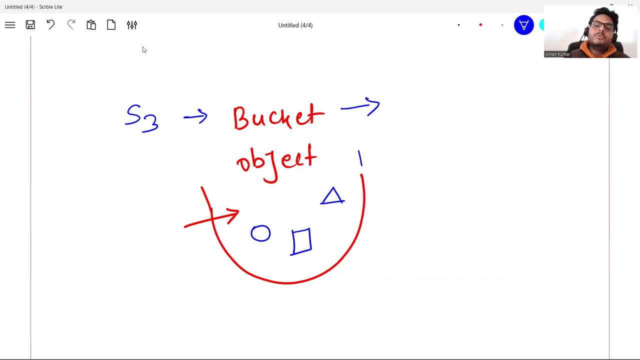 tell one more time: you cannot have. you cannot store file in aws without creating a bucket. you create a bucket first. in this bucket you store whatever you want to store. in this bucket you can store whatever you want. those are called objects. let's see by demo. okay, guys, if you are liking the 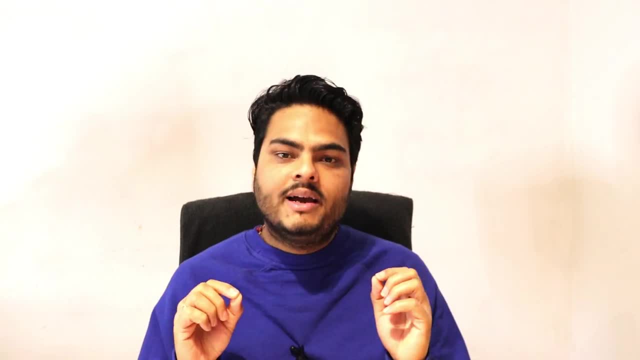 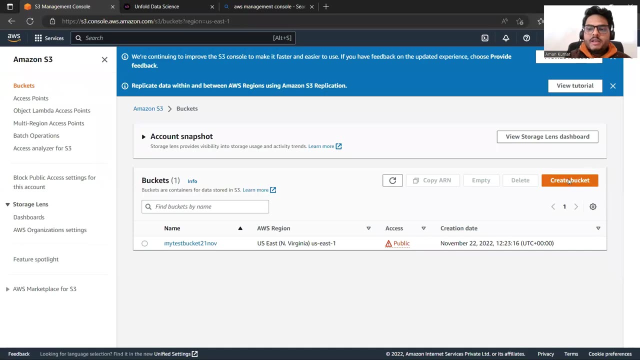 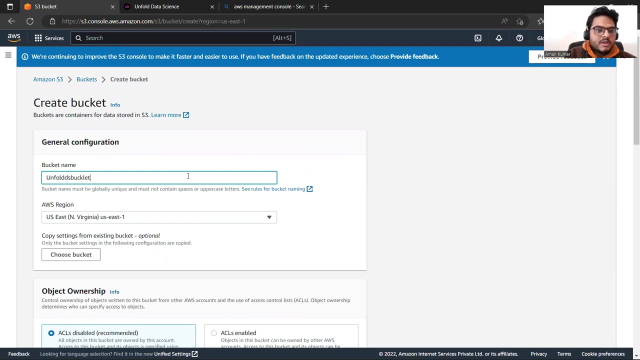 video so far. please don't forget to press the like button and drop a comment saying that you want these kind of videos. so come here. come here and say create bucket, click on create bucket and name here, so unfold ds, bucket, bucket. uh, first let me say this: okay, 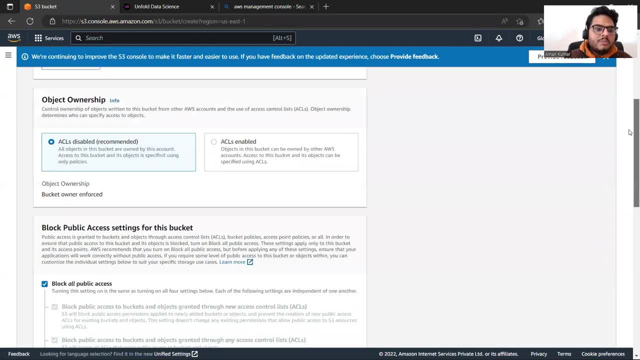 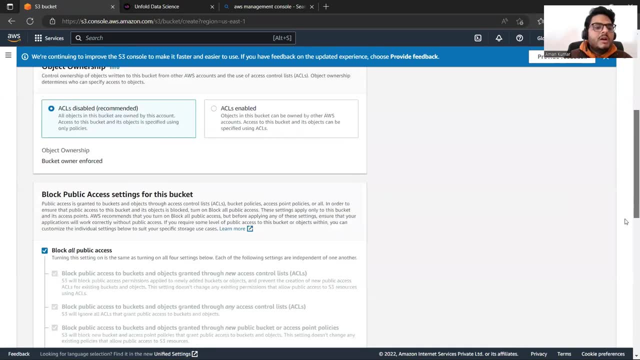 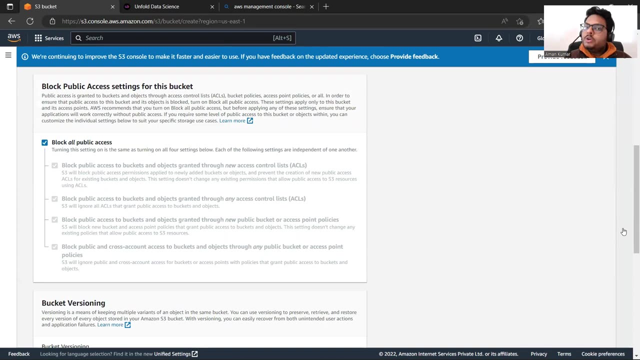 so i'm going to create a bucket for default ds bucket first and i'm not- i'm not kind of uh, doing anything else, i am just going with default settings. now you remember, guys, i told you, uh, i will access this. whatever i am storing in this bucket, i will access this using open internet. 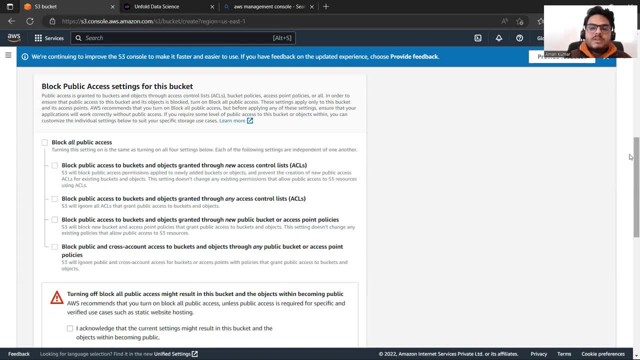 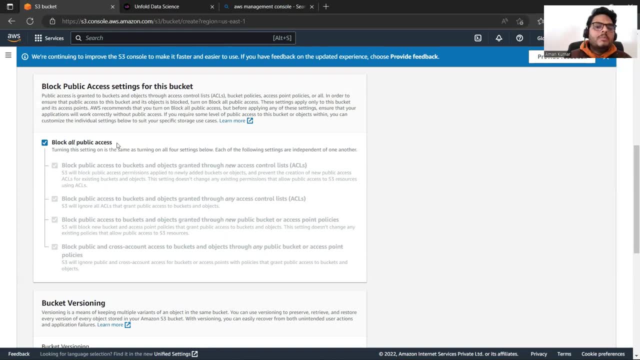 okay, so i will just uncheck this. this is a dangerous thing to do, but i will uncheck this so that public access is enabled. if i check this, it will block all public access. later also i can check in this, but okay, let me change later only. okay, so bucket i am, for now i am blocking all public access. 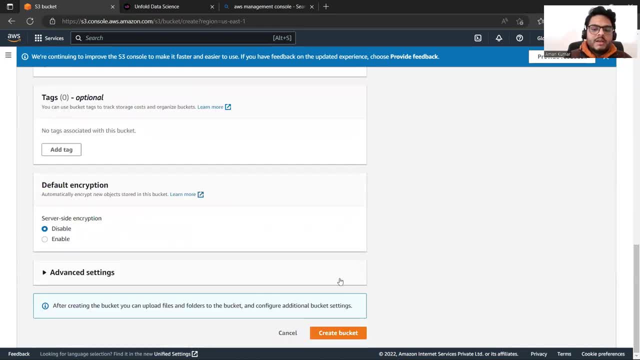 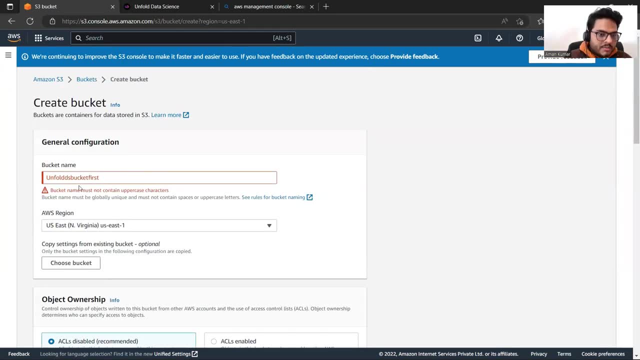 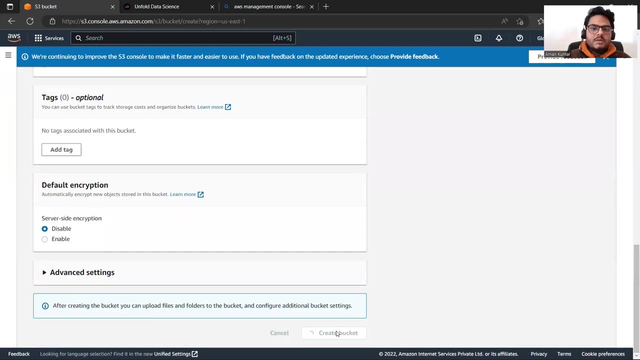 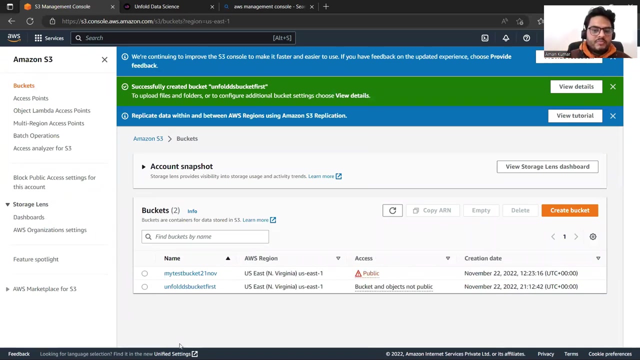 okay, simple. now let's go here and create bucket. okay, what it says? some error. bucket name must not contain uppercase character. okay, fine, so unfold bucket first. let's go here and create a bucket. so what, we are creating a bucket. inside this bucket we can store multiple files. okay, so i will go here and i will upload any file now if i go to my 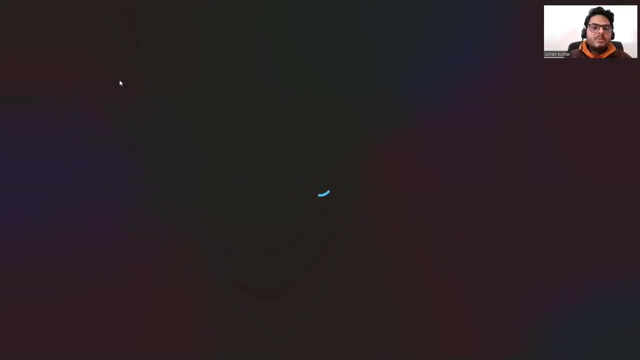 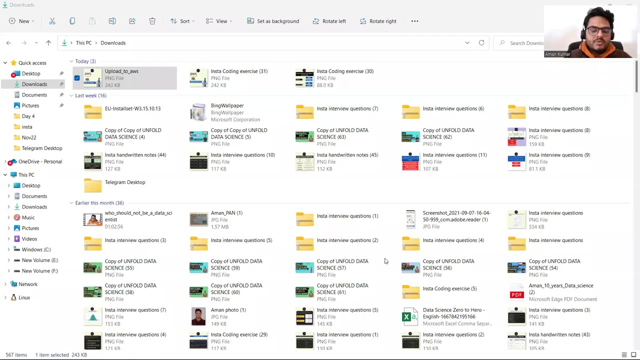 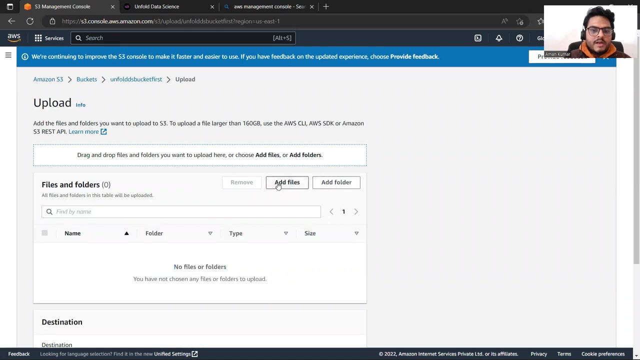 local machine. guys, there is a file called upload to aws. this file okay, and i want to upload this file in cloud now. so see the magic of cloud now, and you can also parallely upload one of your file. add file. add file. go to my downloads. upload to aws. take this: 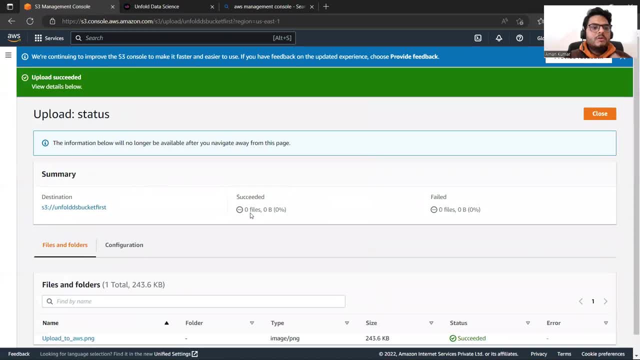 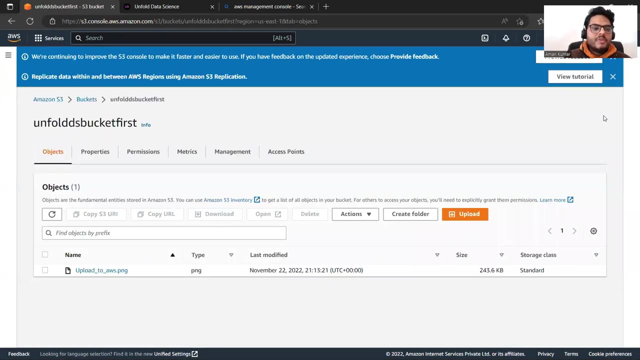 and say upload: okay, uploaded now. so now my file that you saw in my downloads folder is uploaded where amazon s3, which means cloud service provider, okay, and upload status is done. i will say close. now this is my file, guys. okay, in this file there is something known as copy s3, uri. copy s3 i means in the world of amazon. 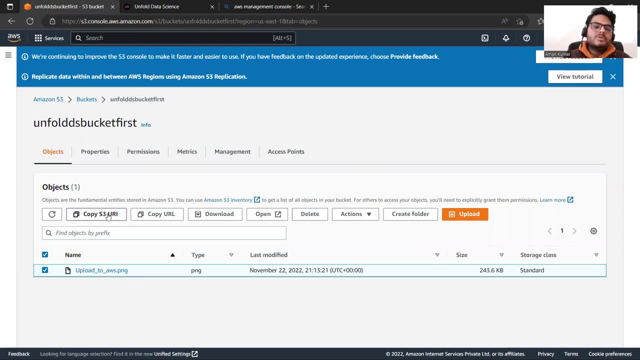 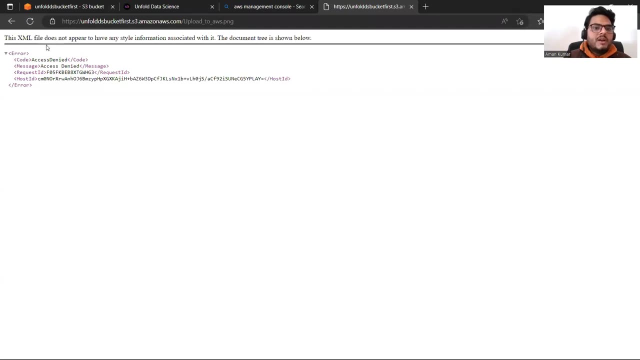 on s3. what is the uniform resource name for this? or uniform resource identifier? okay, and then there is something called copy url. copy url means it will give me a public url. now let's go here and try to paste this. okay, and let's see what happens. see here: the xml file does not have permission. 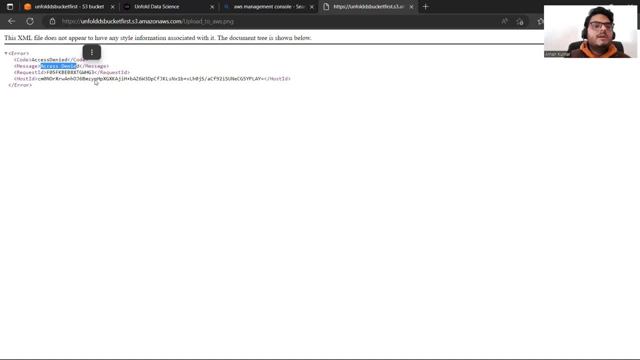 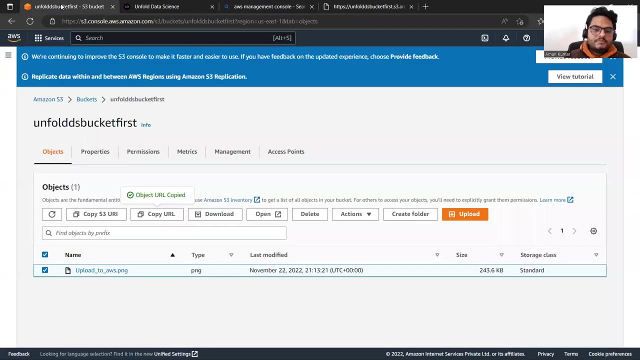 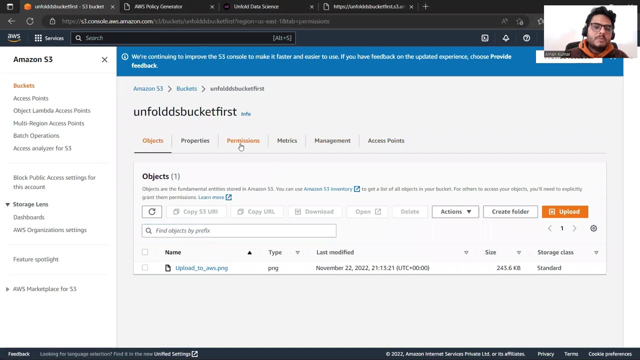 see access denied. do you know why access is denied? because i don't have public access for that file. okay, let's try to go and change it. so another thing we have to do here is go to this new bucket that we have created and go to the permission, and we have to edit the bucket policy. now what is? 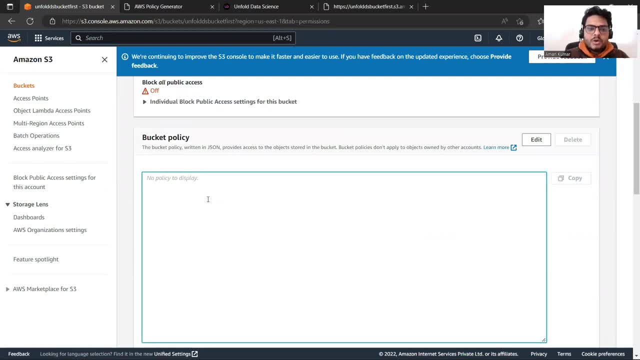 bucket policy, guys, since we want to access it from outside, from open internet. so we have to say to aws that give this access to open internet or make this bucket available to the public. okay, how to do that? this bucket policy is basically a json file, but to a new person it will be difficult to write. 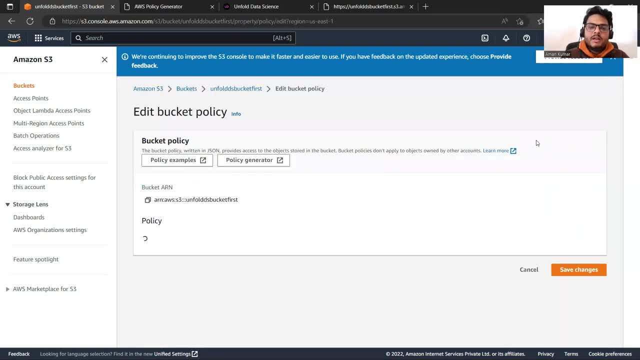 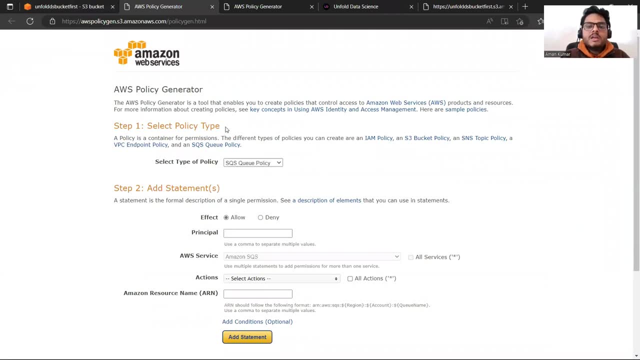 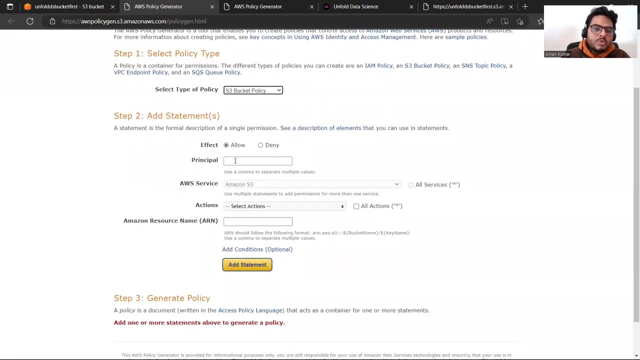 that json file. so there is a very good graphical user interface where you can generate the policy. okay, if you go to policy generator here first say select policy type, so you can go here and say s3 bucket policy, okay. second thing: it comes here what i want to do: i 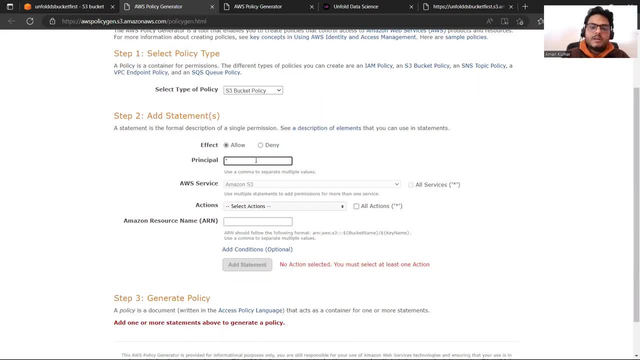 want to allow, okay, and i will say: principal is star. okay, aws, aws. i will say, let it be. uh, this, and here i will say all services, all actions. so amazon s3 is the one one you know in this service we are trying to do okay, so not in all services, amazon s3 service. 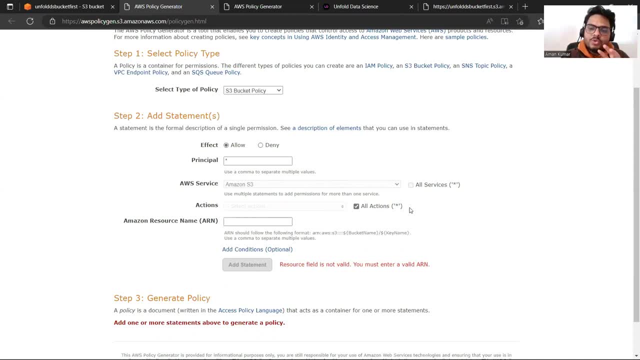 and here action, i will say all action. this is a dangerous thing to do, which means delete the bucket, update the bucket, etc. i am giving a public permission but for showing purpose i can do that. otherwise, what you can do is you can go here and select, you know, get object access, or you can go. 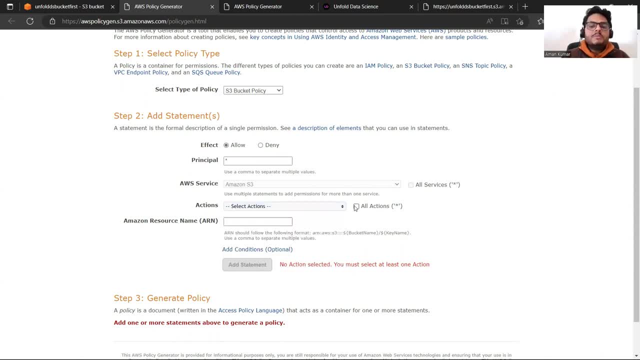 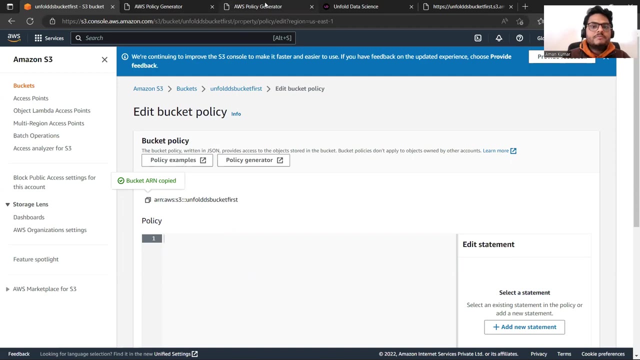 read access or delete access, etc. okay, for now i am saying: add all actions. and then one important thing is amazon resource name. amazon resource name is nothing but your bucket arn, arn. wherever it says arn, it's amazon resource name. copy this and come here to the policy generator, come here to the 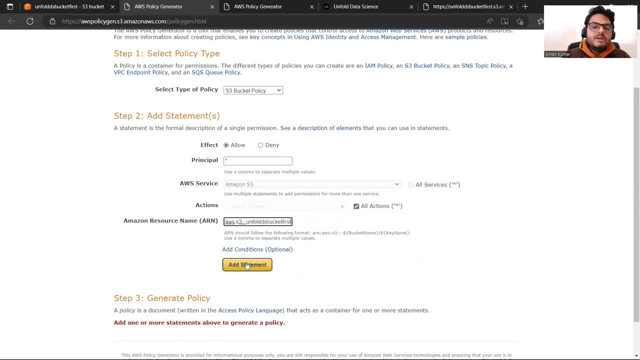 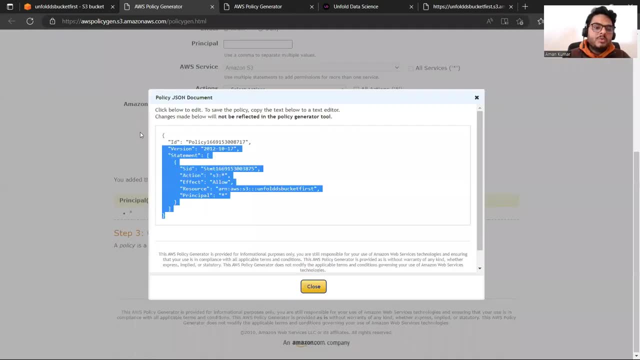 policy generator and paste it, okay. and then you say: add statement. once you have added statement, then what you can do is you can say add statement and then you can paste it, okay. and then you say: you can click on generate policy. it will give you a policy copy. this come here and paste here, okay. 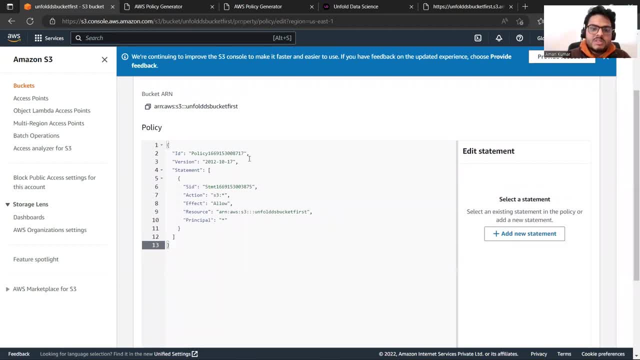 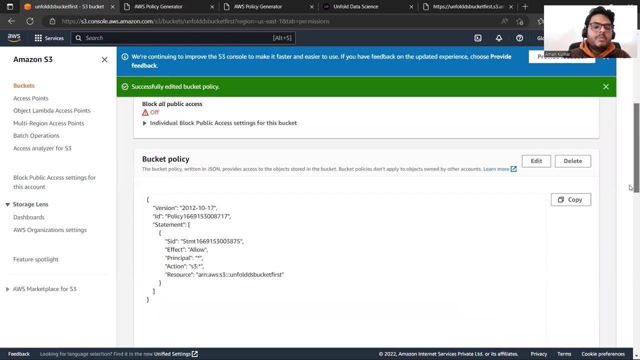 so if you see here what, what is? this is a policy that is, this version version is taking default from my previous policy actually. then statement id, then s3, then allow, then on this bucket and principal register, let me try adding this. okay, so it has got added and now my bucket should be. 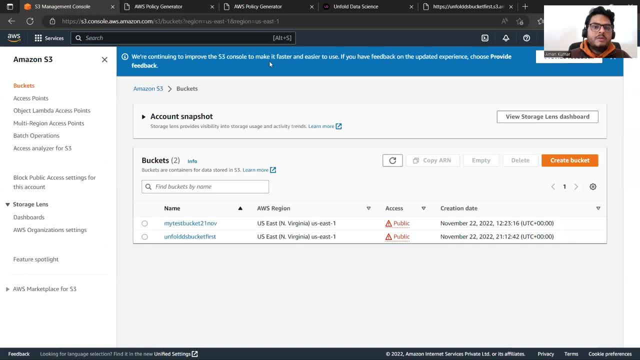 publicly available. let me go here and let me refresh it. it should show me public in in this bucket as well, the other bucket. okay, so you can see it is public now. let me try open this url. let me try refresh this from the open internet. again, it does.